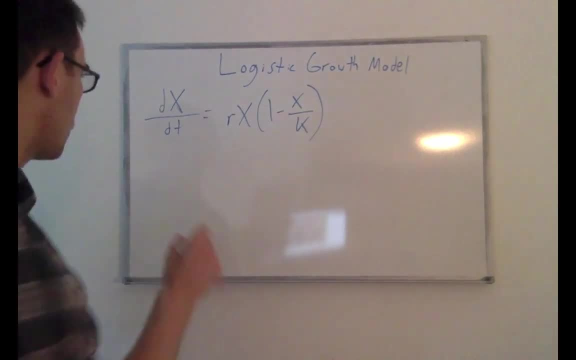 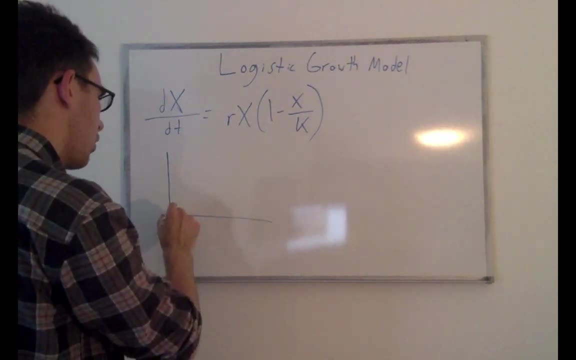 So yeah, a pretty simple model. I'll kind of draw what it ends up looking like. So if you start off with like one cell, it kind of starts growing like almost exponentially and then it like flattens out around this carrying capacity k. 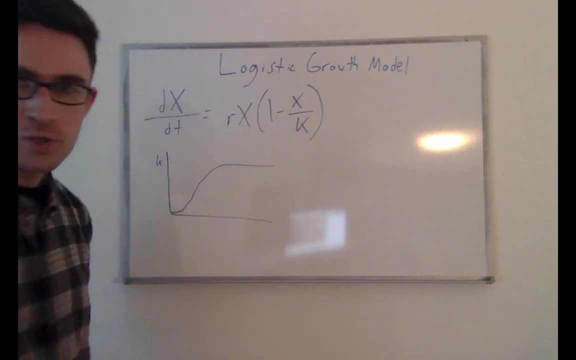 That's kind of what it looks like. Yeah, just pretty, pretty simple, pretty straightforward. So the challenge for this video we're going to use this Markov chain Monte Carlo method 4, is to- is to fit this ODE model to some. 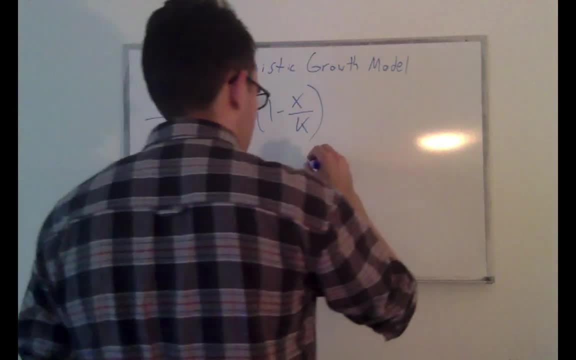 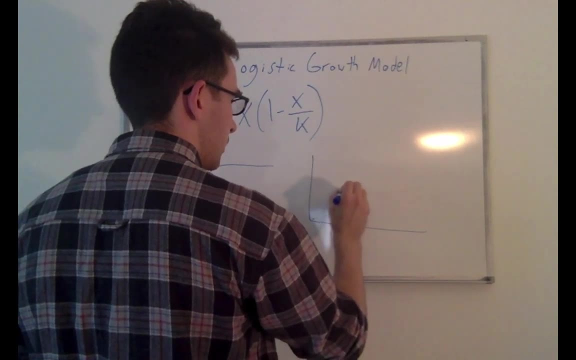 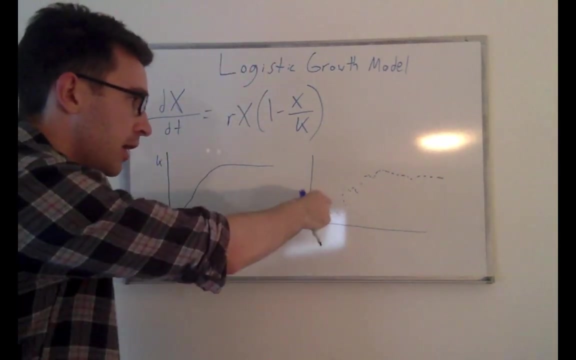 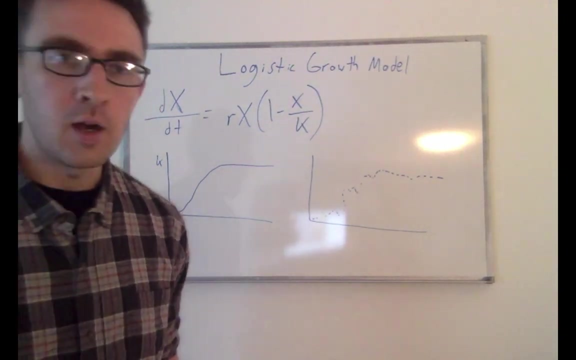 some like actual data set. So basically I'm going to be giving you guys like like a noisy data set that maybe kind of looks like some kind of like simulated like noisy data set, And I actually produced this data set by running a stochastic simulation in Python. So at the end of the video I'm going to show you guys what parameters for r and k 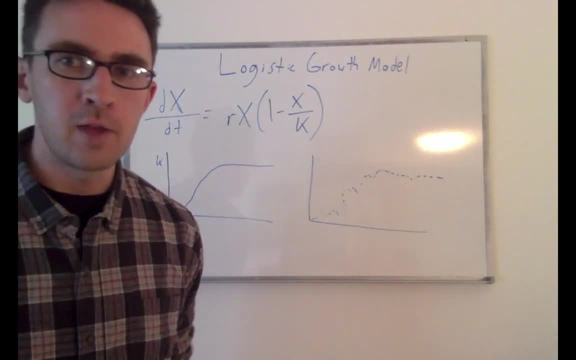 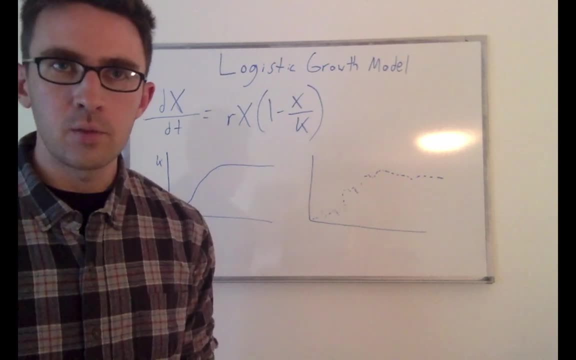 I actually used to generate this like fake data set, But that's going to be at the end of the video, So what we're going to do before then is we're going to try to use this Markov chain Monte Carlo method to fit the parameters to the data and 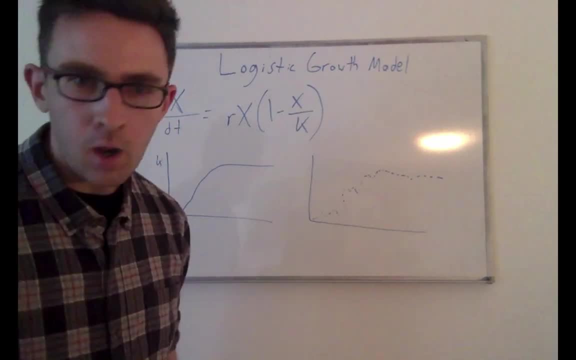 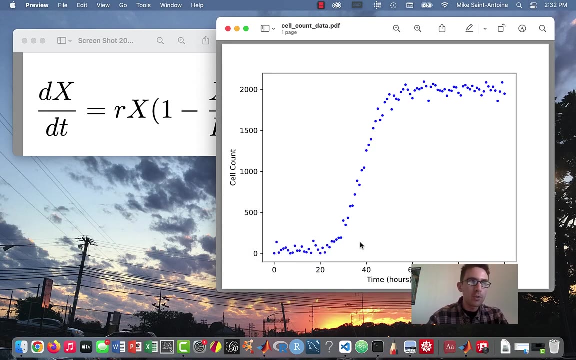 estimate these parameters. That's going to be kind of the goal for this video. Okay, so let's get into the code now. Okay, guys. so this is. this is like the fake data set that we're going to be trying to fit- fit our ODE model to. 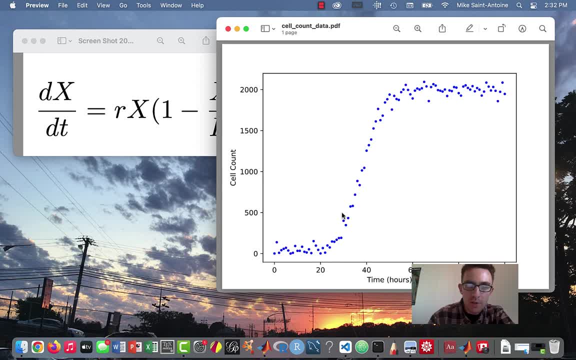 So again, I kind of just produced this set, this data set, by doing a stochastic simulation in Python and I chose some like r and k parameters to use for this, and at the end I'll show you guys what the actual parameters I used were. 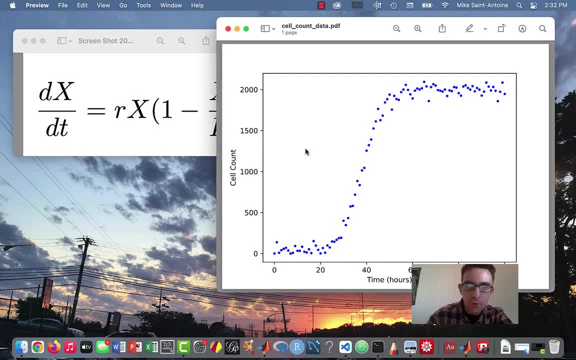 But for now we're just going to try to fit this ODE model to the data and just to remind you guys again, like the purpose of parameter estimation is to try to find the values of r and k that allow this model to most closely fit the data set we have. So yeah, this is what the data looks like. 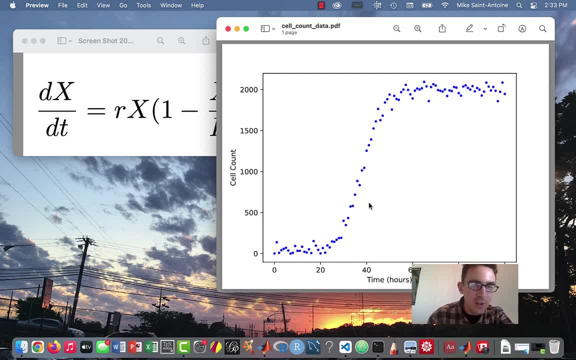 If we're like, if we want to kind of like cheat and take the easy way out here, we can kind of already see, like, what the carrying capacity is. but let's not, let's not do it visually, Let's try to actually like, write this Markov chain, Monte Carlo method properly. 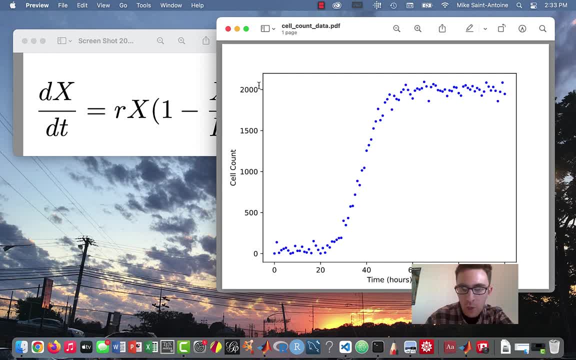 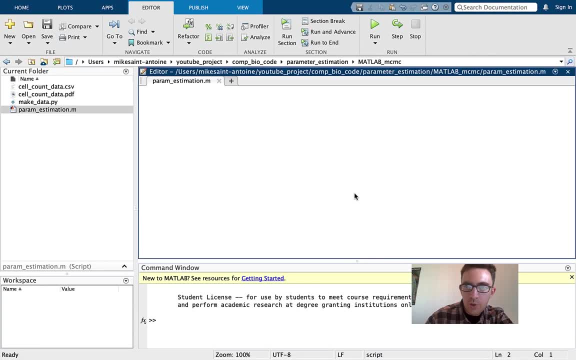 and see if, see if it can figure out the parameters itself rather than just kind of looking visually at what the carrying capacity is. But yes, this is what the data looks like. I also have it in CSV format here. Like usual, I'll put this all up on my github if you guys want to download it and try it out yourself. 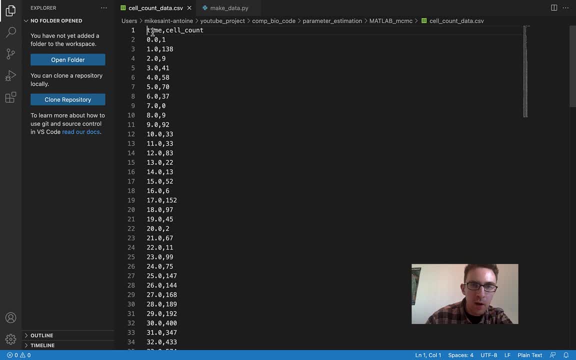 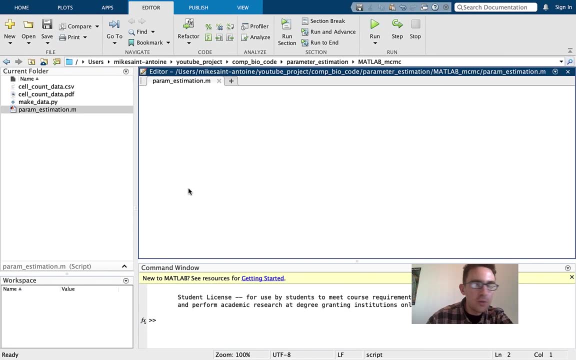 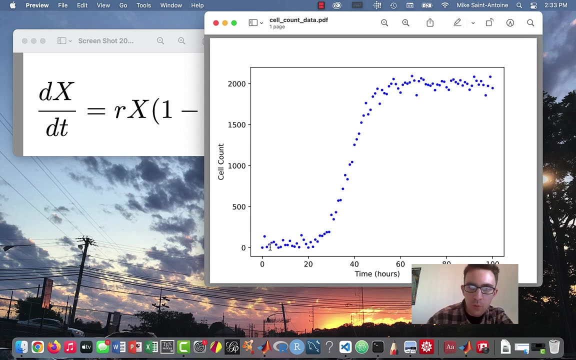 Yeah, so just the CSV format it has. it has a column for the time point and it has a column for the cell count at that time point, and we're kind of assuming here that there's some like experimental and and like biological noise here. So there could be like measurement error as well as like 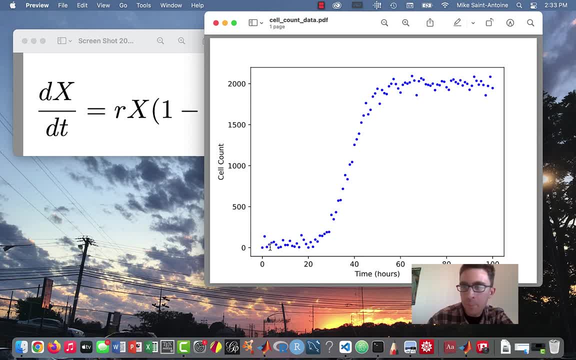 cells growing, cells dying off and you know, just just some noisiness in the data. But yeah, so we want to use this Markov chain Monte Carlo method to search through the parameter space and try to figure out which values of R and K. 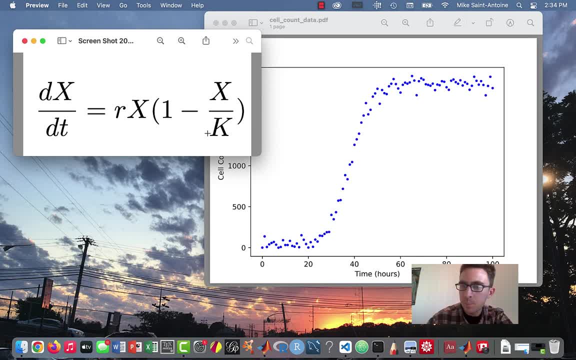 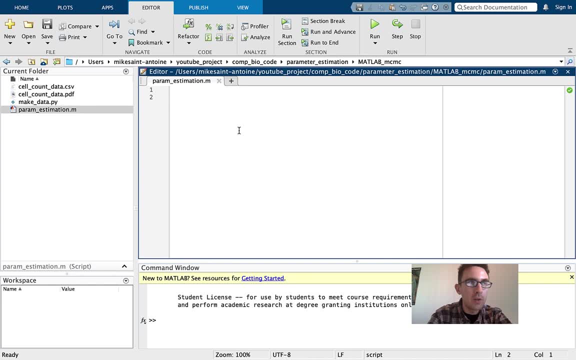 cause this OD to best fit the data. Okay, and we're gonna be using MATLAB for this, and the reason I'm using MATLAB here is just because that's that's what the request was. One of my viewers wanted to see how to do this in MATLAB. 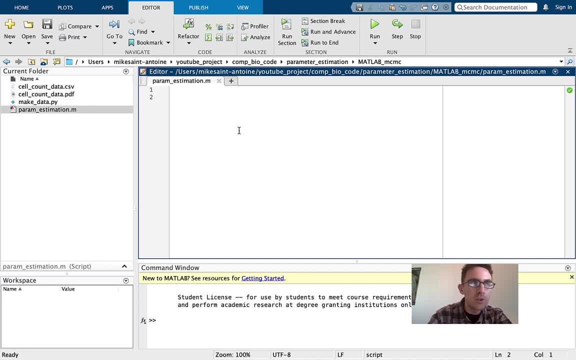 Personally, I'm not a huge fan of MATLAB and if if I, If I was doing this myself, I would probably use Python. But I recognize that people, especially in academia, a lot of people do use MATLAB, So it is good to. I think it is good to be like making some like tutorials on MATLAB too. 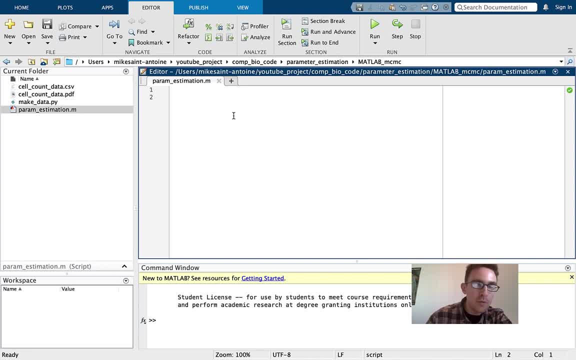 Just because I know people use it, But disclaimer for this video. So in order to do all the stuff I'm going to do in this video, you need to not only have MATLAB, but you need to have the statistics and machine learning toolbox installed. 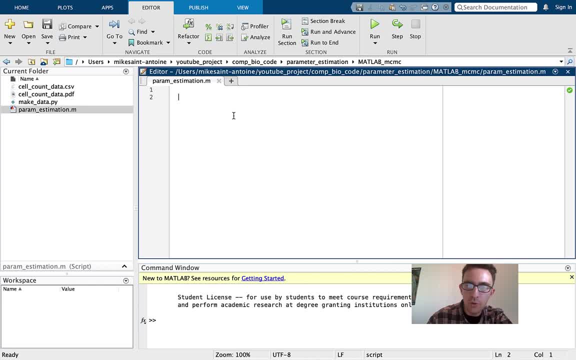 So if you don't have that installed, you're going to need that to be able to do all the stuff in this video. Yeah, again, that's kind of one of the things I don't like about MATLAB. It's like you need to pay for these like extra things to be able to do a lot of the like basic stuff. 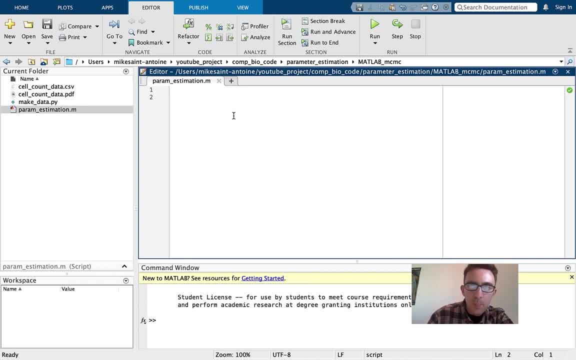 that you could do for free in another language. But yeah, I mean, that's just how it is, I guess. Okay, so just like, first things first, let's just read in the data and just make sure we can get the data in. 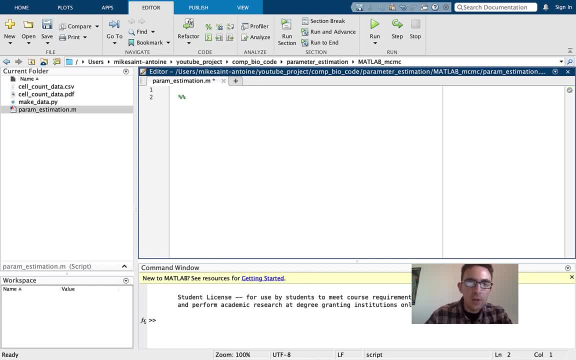 Okay, so to do this, I'm just going to make this section- Yeah, let's call this read in CSV data. I'll just call it, maybe something like like an abbreviation for experimental data, CSV read and then this, this file: So cell count data dot CSV. 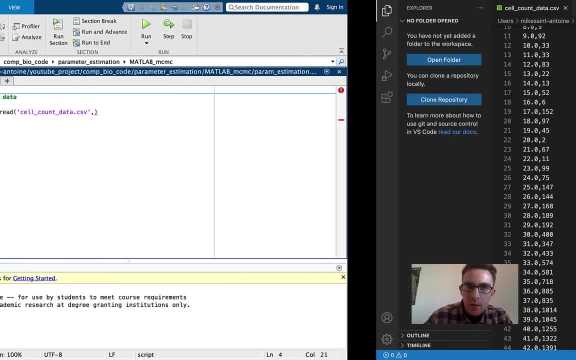 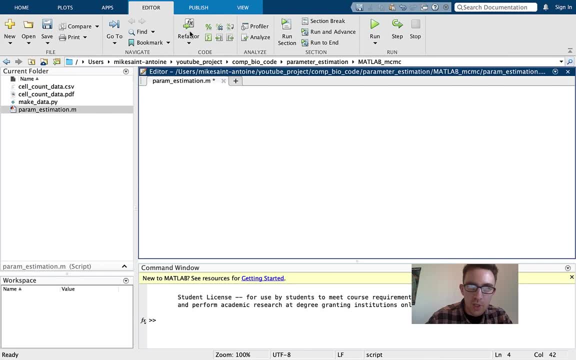 And this has a, this has a heading. So we want to, we want to, we want to let this, the function know that there's a. the first row is a heading, So to basically skip over the first row. So I'm going to put a one here and then a zero, because we're not, we don't have like a column index. 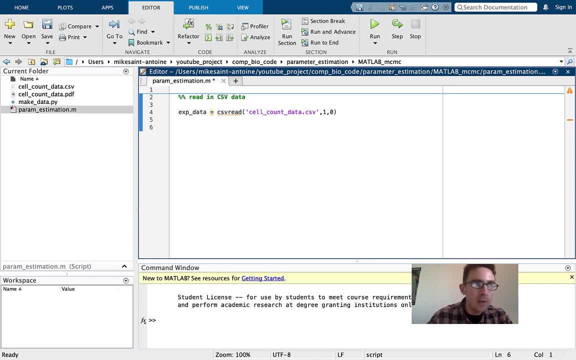 Okay, and we're basically going to see if we can read this in and then plot it and just like make sure we can like recreate this, Something like this pot we have here. I just want to try to like plot out this, plot out this data and make sure we can, you know, read it and read it in properly. 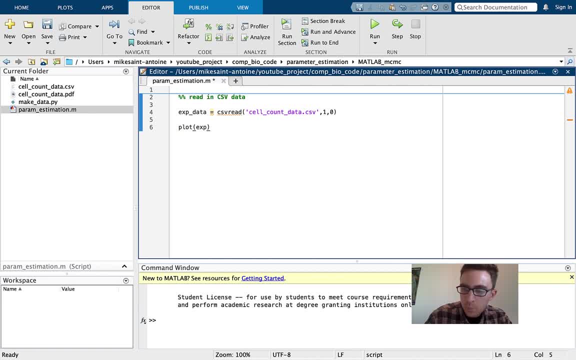 So I'm going to plot X data Again. the first, the first column, is the time points. So we're going to plot all of the rows in the whoops- I have this backwards- All of the rows in the first column. That's the time points. 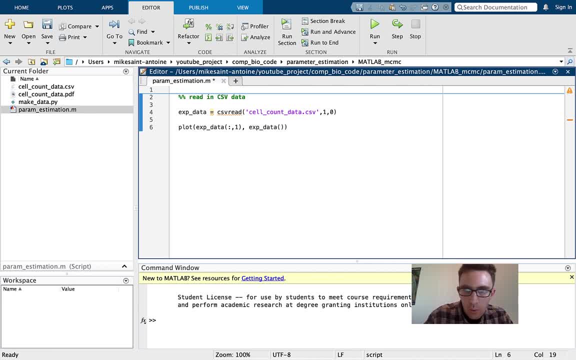 And then All of the Rows in the second column, That's the actual cell counts. So yeah, let's just run this and see if we can just like read this data in and plot it properly. Whoops, forgot. So my colon there. 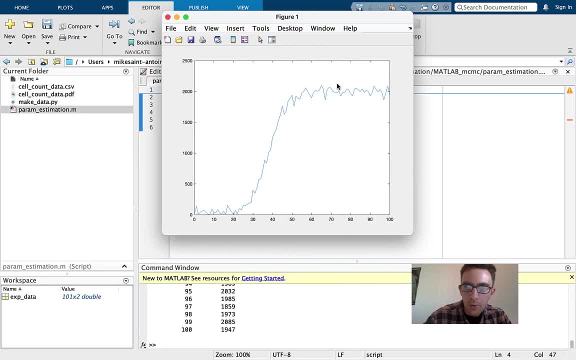 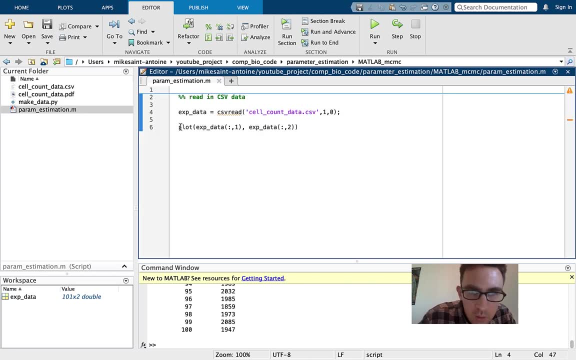 Yeah, looks like it, looks like it right in, Okay, And plot it Okay. Yes, we're good. We're good so far. So I'm just going to comment this out and then we'll proceed on. So again this: I don't want to make this into like a big complaining about MATLAB video, but you can even see, just watching this, like it's, it feels it's slow and like laggy and I don't know. 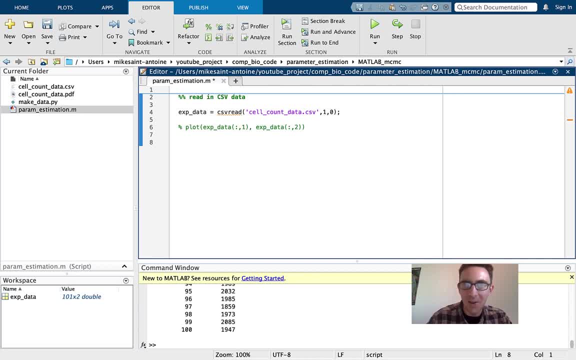 I don't make this into like a negative video about that, But, but yeah, I'll just keep my opinions on myself for now. Okay, But now that we've read in the data that the next part is going to be actually coding this Markov chain, Monte Carlo method. 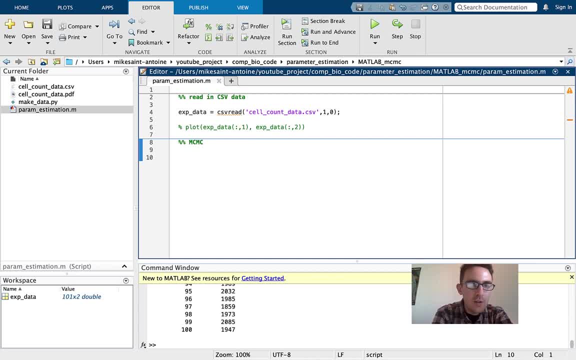 So basically, like the Markov chain Monte Carlo method is it's a way of searching around. It's a way of like searching around a parameter space that corresponds to a probability distribution. So basically, like if you guys have watched any of my like previous like parameter estimation and machine learning videos, like normally we have some kind of loss function that we're trying to minimize, that like measures how far off the model is from the data. 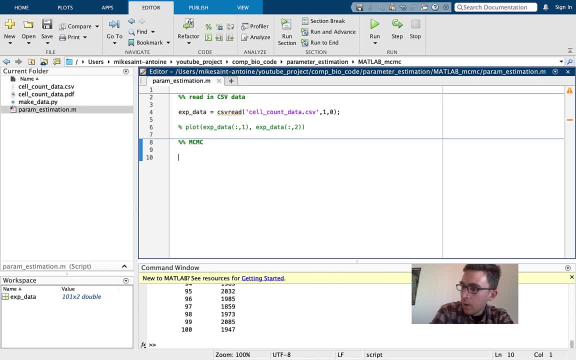 And we want To, like minimize that loss function. with Markov chain, Monte Carlo, It's kind of the opposite. We're actually going to have a log likelihood function that is going to measure how basically, basically how likely we would be to observe the data if some, if some given parameter set was actually the true underlying parameter set. 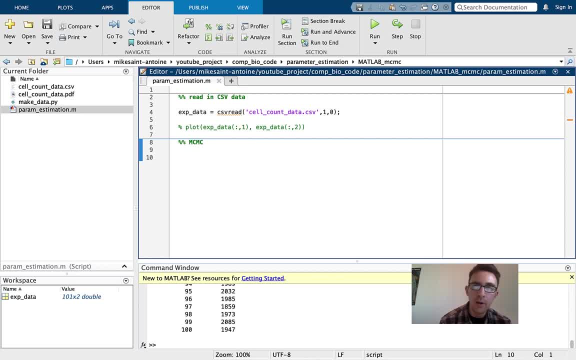 So it basically measures like the goodness of fit of a parameter set to the data, And so, instead of like Minimizing a loss function, like like we do for like least squares or something like that, we're actually going to be trying to maximize a log likelihood function. 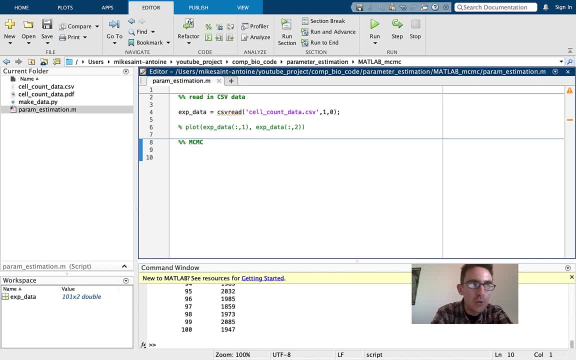 And basically the Markov chain. Monte Carlo method is just a way of like searching around the parameter space And an advantage to it is that it lets us incorporate some prior distribution we have about the parameters. So in this video I'm going to be assuming like a worst case scenario where we don't have any. 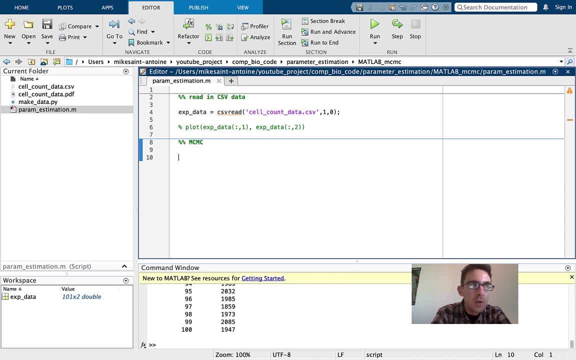 Like prior information about the parameters. but you guys are going to see that we're going to be, like, generating the guesses based on a prior distribution. So if you did have some prior information about what you thought the parameters might be, you could incorporate that prior information into this, into this algorithm, and then, like, search through the parameters in a way that, like, incorporates that prior information. 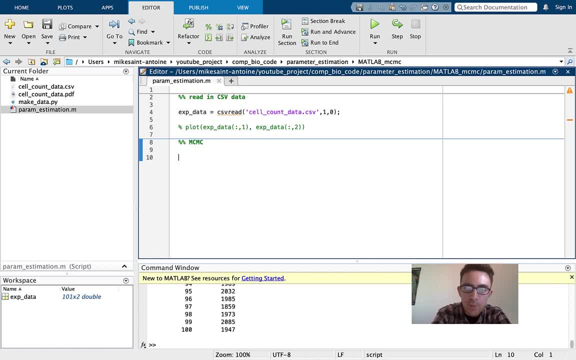 And the goal here is to get a posterior distribution. So if you guys are familiar at all with like Bayesian statistics, You have a, you have a prior distribution and then you like incorporate some information from some data and then you come out with a posterior distribution that includes that new information you got from the data. 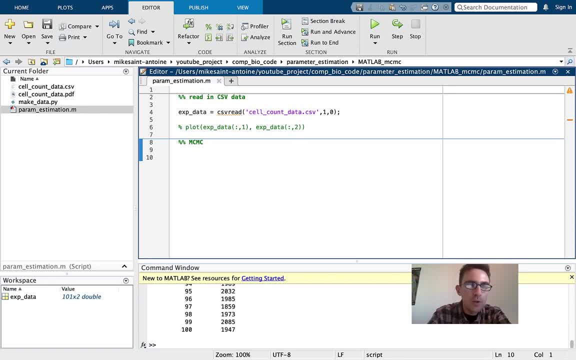 So that's that's going to be. what we're trying to do here is just like have a prior distribution for the parameters and then incorporate our information from our data and then come out with a posterior distribution of like what we think the parameters are OK, so let's get started writing this code. 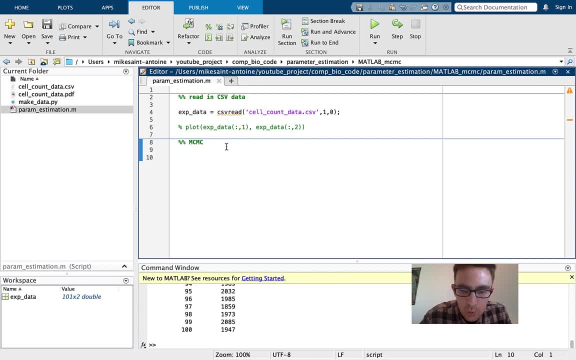 Oh actually, yeah, sorry. Before we even get into the actual writing, the writing, the MCMC, we need to define some functions we're going to be using first to be able to even, like, write the rest of it. So I'm actually going to be a little bit lazy here and just copy and paste in some of these functions. 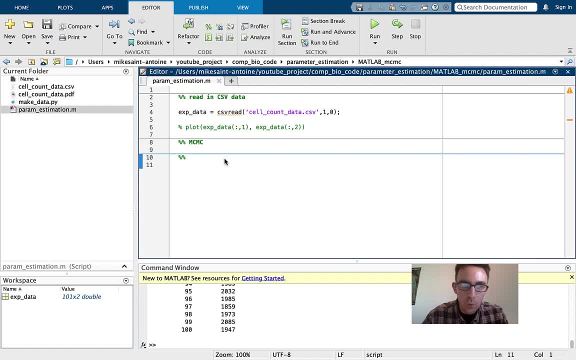 But then I'll, then I'll tell you. I'm going to tell you guys, like what, what they're all doing. But yeah, just in order to save time, I'm going to be a little bit lazy and just copy and paste some of these in. 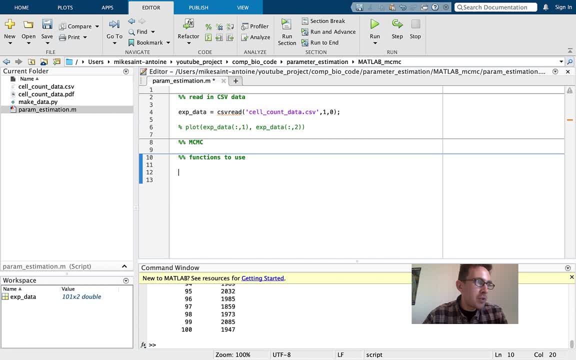 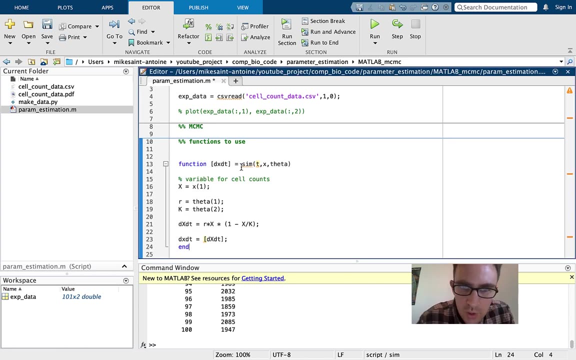 Yeah, it's called like Functions to use. So the first function is just going to be the function that is going to be our ODE model And we're going to use this to like, simulate the ODE using various parameter sets. So, yeah, I'm just, I'm just calling this function sim for now. 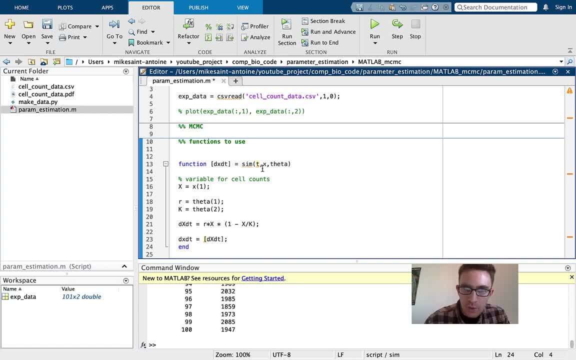 It's just going to be like our ODE simulation. It's going to take X, which is going to- I mean, in this case we only have one variable, But if, like X will actually be like an array. And if you, if you had more than one variable. 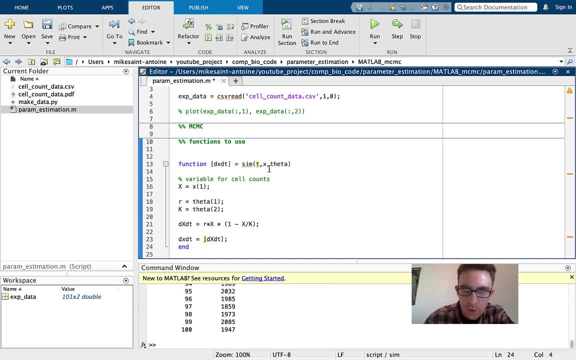 You could store like all the variables in this X array and kind of unpack them. But for here I only actually have the one variable on capital X. So I'm really only unpacking this one variable here And then we're going to have this, this other array. 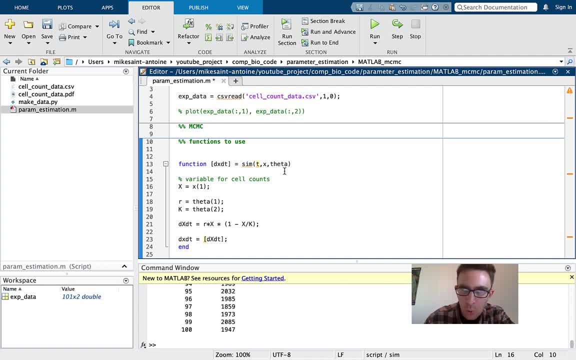 I'm just calling theta. That's just kind of a convention. You could call whatever called params, call it, you know, call it whatever you want. But I'm just going to get data for kind of a convention. Theta is going to be, is going to be what's going to pass in all of our parameter values. 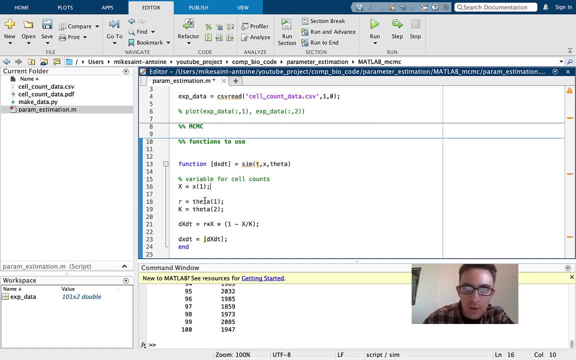 So I'm just going to pass in these parameter values for R and then K- It's kind of like unpack them out of this theta array here- And then I'm just going to calculate this value for DXCT, which is going to be R times X, times one minus X over the carrying capacity. 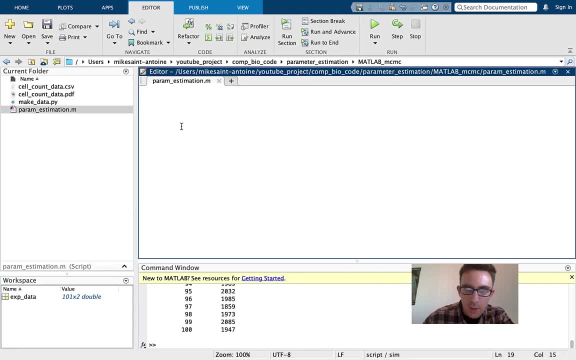 Again, just our, our ODE here And then, and then just going to return that out of this function. Basically, this function is just going to be what's what's going to allow us to Simulate this ODE for different, different parameter sets. 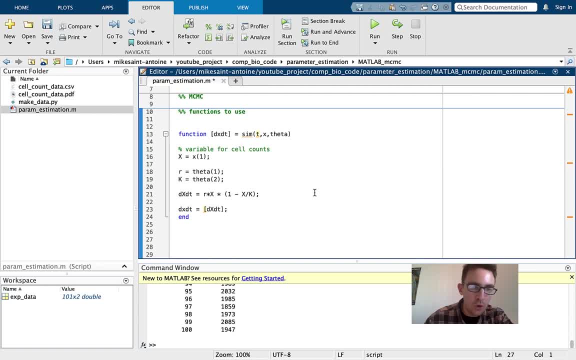 We're going to be passing in And just remember, just remind you guys again, the goal is to like, try out different parameter sets and then try to see which one produces results that most closely match the real data. So, yeah, that's our first function we're going to be using. 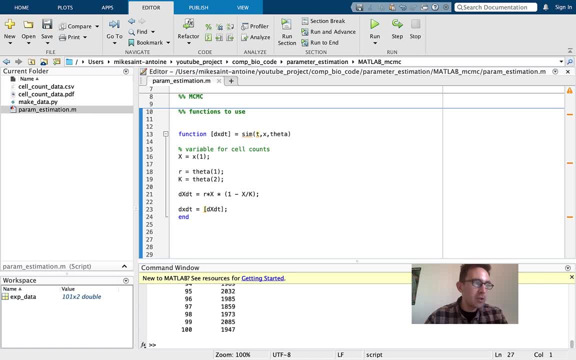 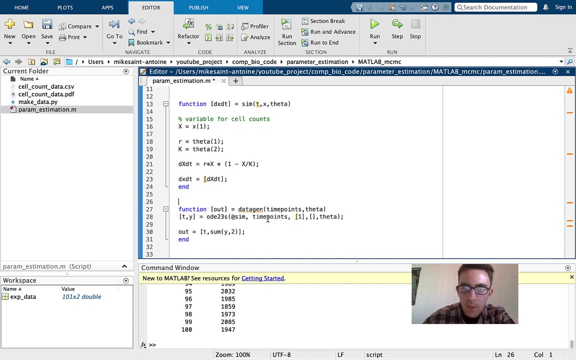 Again going to be a bit lazy and also copy and paste in the second function, Second function here. So this function I'm calling data gen And this is basically Just like passing in some time points and passing in a parameter set, again calling the parameter set data. 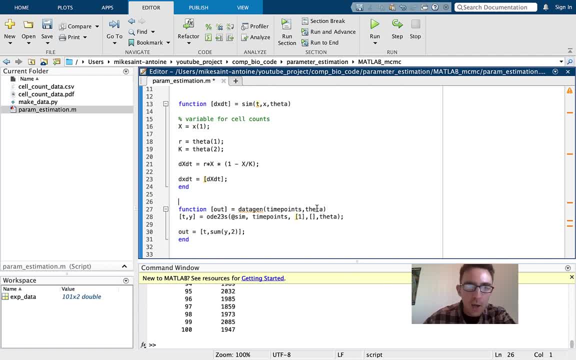 So basically, you just pass in some time points, pass in some parameters and then you just simulate the ODE You you call this SIM, the SIM function here, and use the ODE 23S solver built in built in MATLAB solver here. 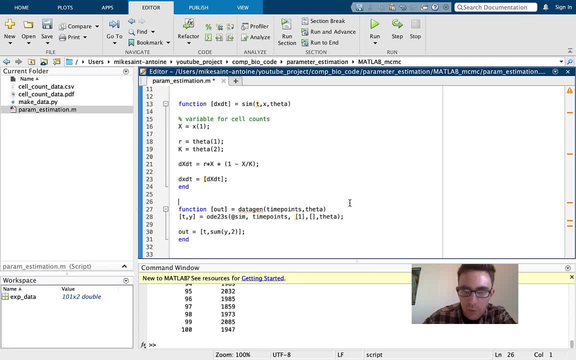 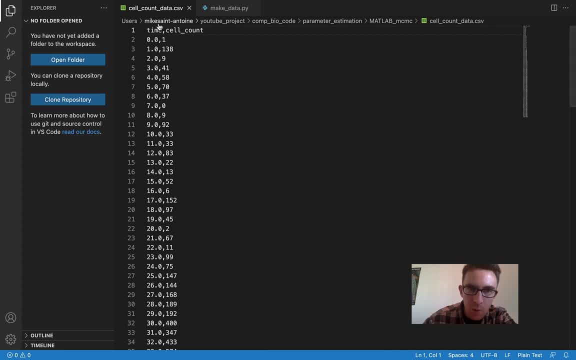 You basically just solve the ODE at these time points for this parameter set. Oh, and the initial condition too is just going to be Starting with one cell. I'm just getting that initial condition because at time zero we have one cell that we're starting with, so that this: 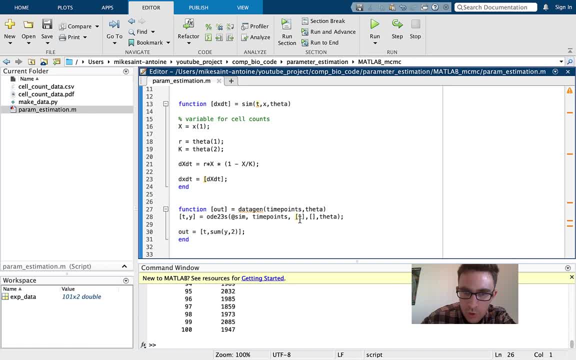 Yeah, this here is just the initial condition of starting with one cell. Yeah, so basically you just pass in the time points you want, you pass in the parameter set you want to use and then you solve the ODE for that parameter set at those time points. 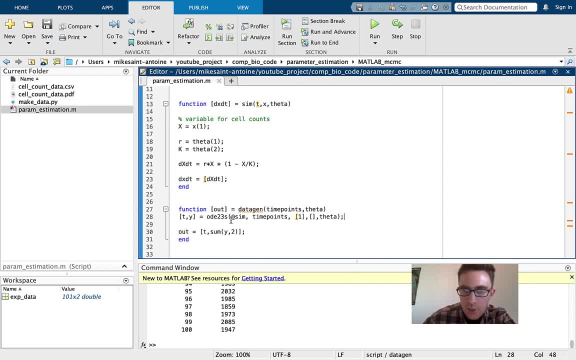 And then you're just returning the time points and the cell counts that you solve You got By solving the ODE's. So yeah, pretty straightforward. We just have our ODE function and then this other function that it solves the ODE's for some time points and some parameters. 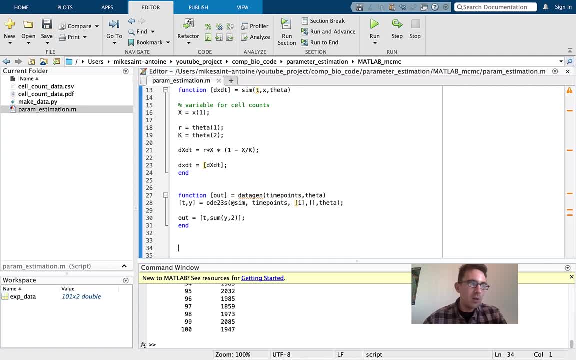 OK, so there's one more function we need, and this one is going to be a little bit more complicated, but still still not too bad. So this is going to be our log likelihood function And again, just going to be a little bit lazy and copy and paste this in. 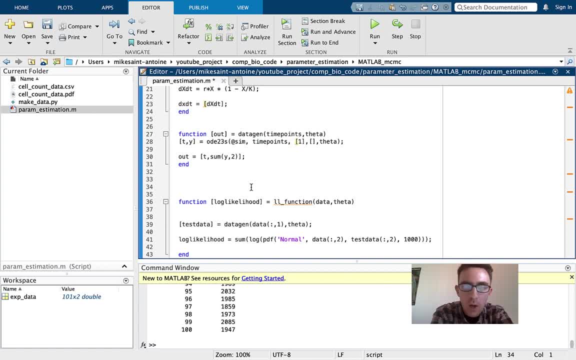 So yeah, Basically, our log likelihood function is a measure of: is basically, is basically a measure of the likelihood of observing, observing the real data, given that the underlying parameters that that we've picked for this test parameter set are actually the truth. Like, given those parameters, what's the likelihood of observing this real data set? 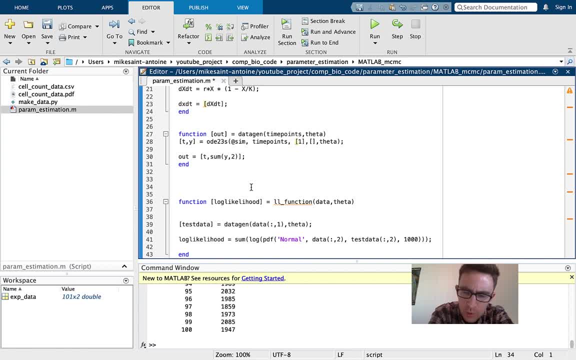 And so it's basically like, if you don't want to think too much about the probability, Just think of it as like a goodness of fit score. It just matters like I mean sorry, it just measures like how good of a fit are our chosen parameter? set is to the data. 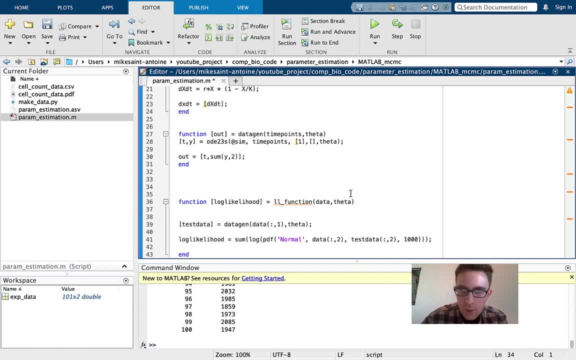 So basically, you just, you just pass in the real data and you pass in a parameter set And then the first thing it does is it calls this data gen function And it just, it basically, just like it just solves the ODE's at the time points of the real data for this parameter set. 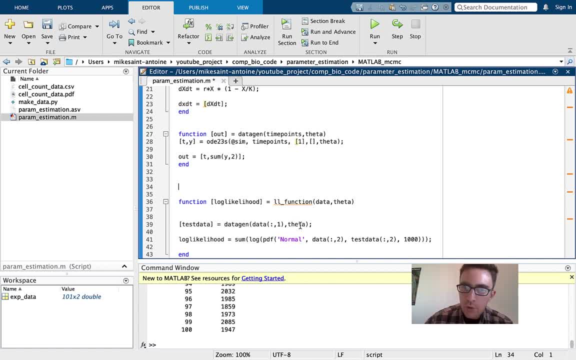 Right, Passing in again, just calling it data for convention here. And you, you generate this like test data set, just solving, solving the ODE for this parameter set at these time points. Again, just the first column of the data is. that is the time points. 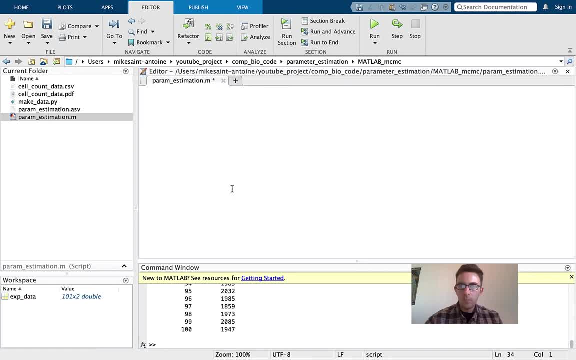 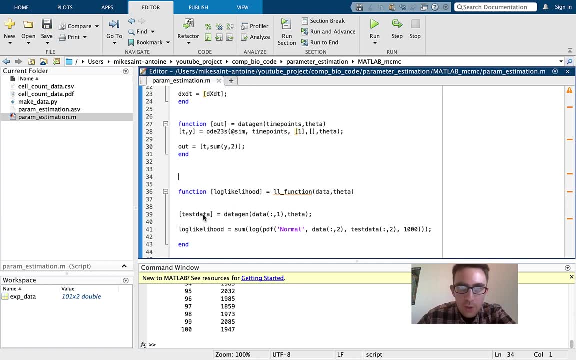 Just remind you guys, your first column is the time points. So yeah, just just generating a test data set, basically just saying, like, what does the ODE predict? Like, yeah, just what does the ODE predict For the cell counts? given some time points and given some, some parameters, we're passing in. 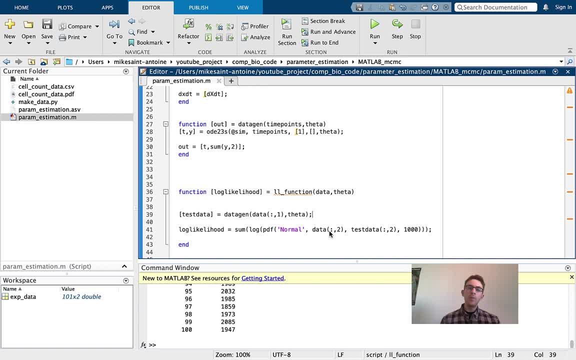 And then, OK, this part is the part that's kind of confusing, but it's really not so bad if you kind of like go through it step by step. So, basically, this is just this: just computing the log likelihood score, That's just measuring how, how closely our test data matches our real data. 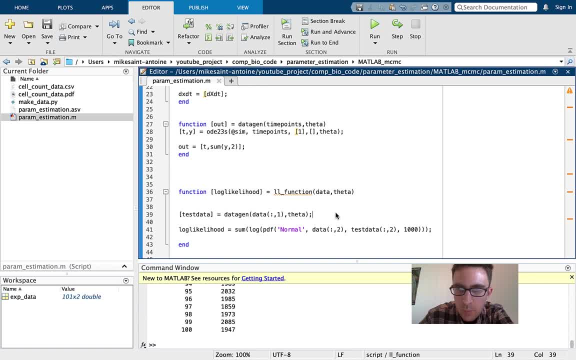 And again, just this is basically just a measurement of how closely the parameters That are used to generate the test data match our real data. Yeah, So, basically this: this is using the PDF of the normal distribution and just like getting the getting the PDF score, getting some P value here of of like, for each one of the real, each one of the real cell counts at each time point. 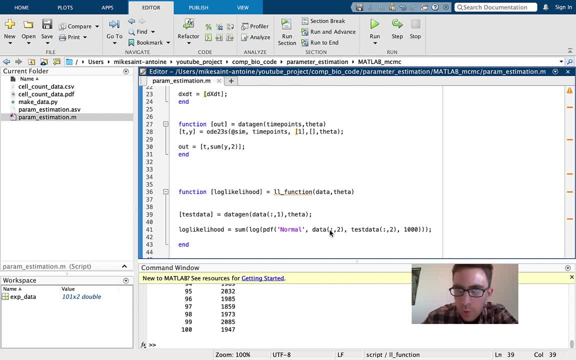 Just getting getting the P value of, of observing something at least Extreme as that real cell count and like what that P value would be if the mean of this normal distribution was the ODE predicted cell count at that time point for that parameter, set with a standard deviation of- I just said a thousand for here. 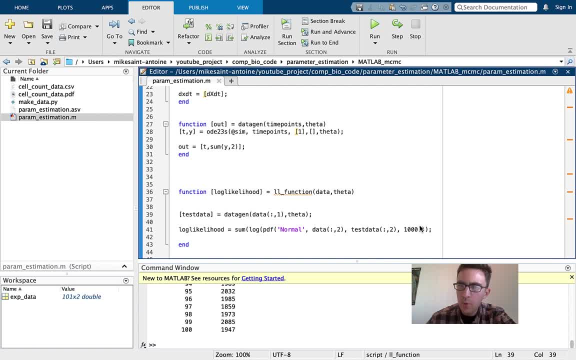 This is kind of like a bit of a shortcut on the theory, because for one thing I'm just assuming a normal distribution here. We don't actually know if if this really does follow Normal distribution. So this is a bit of a shortcut with the theory of this. 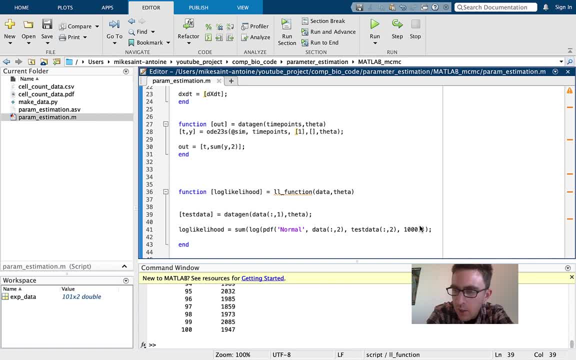 So this part isn't, it's not one hundred percent airtight from like a, from like a probability theory standpoint. I am taking some shortcuts. I'm just assuming a probability distribution and assuming some deviation of of a thousand. You guys could play around with this. 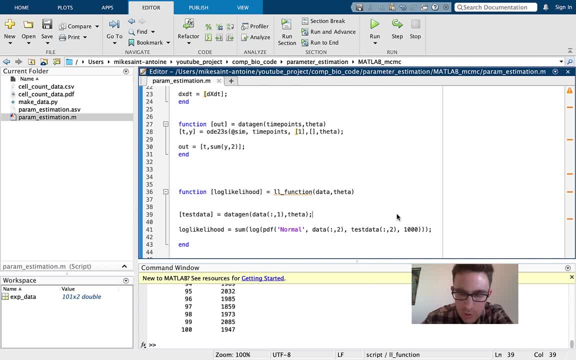 Try out different trial, different distributions trial, different standard deviations. The important thing is that you're using The mean of the distribution, like the mean should be the predicted cell count that the ODE predicted given, given the the parameter set we passed in. 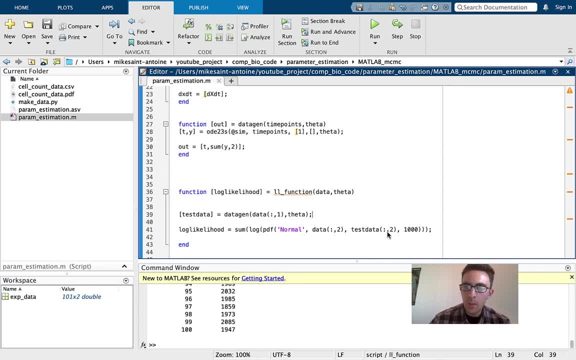 That should be the mean And then the the test data point that we're trying to generate a P value for is the real data, like the real cell count at that time point. So again, this might be a little bit confusing, but basically. 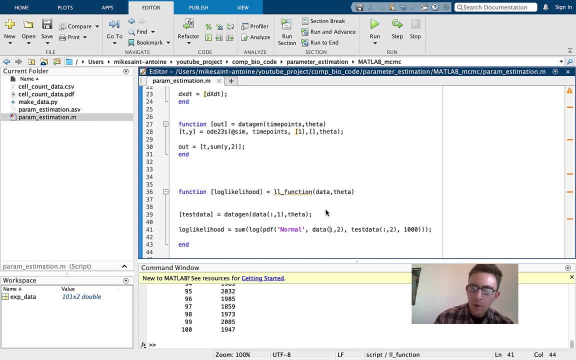 It's just like for each, for each data point we have. we're just trying to get some P value of observing that data point or something at least as extreme as that data point If we assume like a normal distribution with the mean of the ODE, predicted cell count and a standard deviation of a thousand. 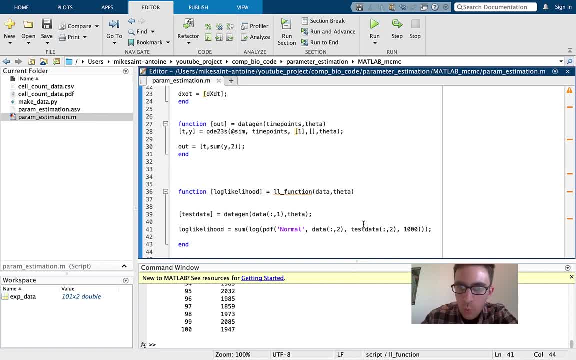 So this is giving us like a column vector here, because we're getting one P value for each data point we have. So the next thing to do is, if you wanted to combine all these P values, you would have to like multiply them all together. 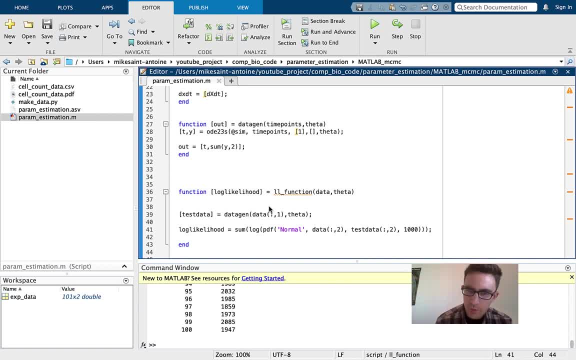 But that's. that's not going to be computationally feasible, because that will give us too small of a number. So what we want to actually do is, instead of like multiplying them all together, we want to take the natural log of all of them. 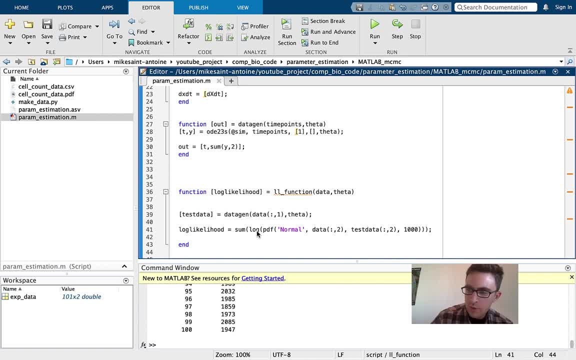 We want to just take the natural log of all of these P values, And that's that's what we're calling it: A log likelihood score Instead of just a likelihood score. we take the natural log of all of these, of all of these individual P values, and then we sum up all of those logs. 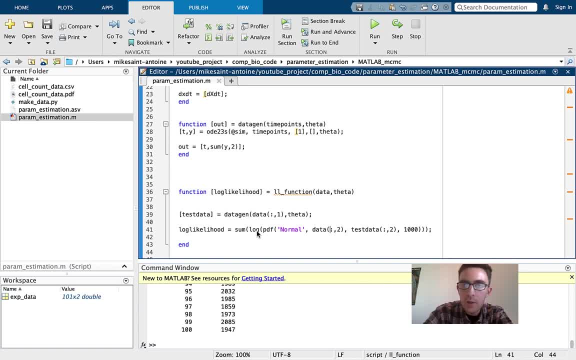 So basically this is just going to be summing up a bunch of negative numbers And basically, the the more negative the number is that we end up with, the worse a fit our, our parameter choice was, and the the closer to zero. So this log likelihood score is meaning the less negative it is or the higher it is, that that means it's a better fit. 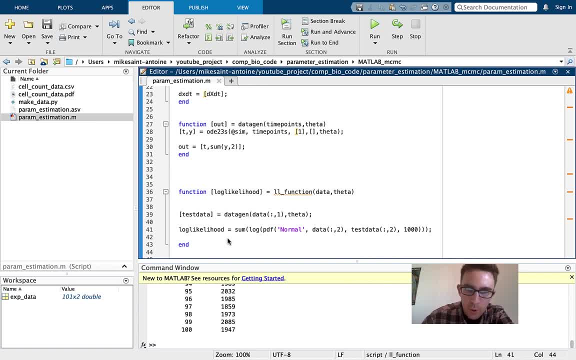 So, basically, this is going to be some like some negative number and we want it to be as close to zero as possible. Basically, we want it to be as like, as as high, as as close to being positive as possible, And the lower it is, the more negative it is, the worse of a fit it is. 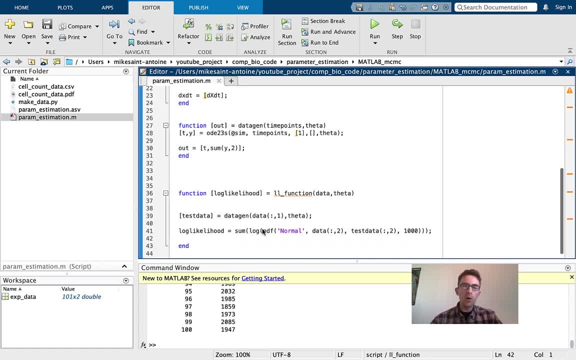 So yeah, these are the functions we need. again, Maybe this part is confusing And again I acknowledge that I'm taking some like shortcuts on the theory here. just assume, assuming a normal distribution and assuming some standard deviation, just to make the make the calculations work. 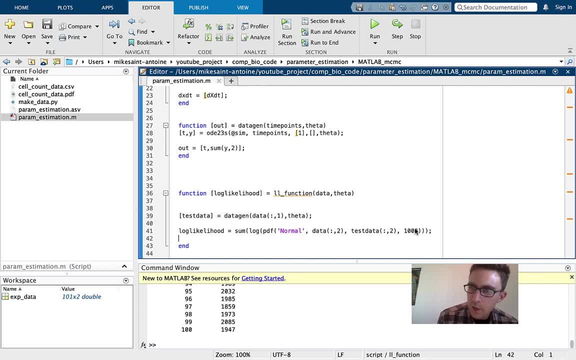 My philosophy is that it's so. it's okay to take shortcuts, like to the extent that you still end up with the right answer. So, like, my way of thinking about this is that, as long as we still end up getting the right parameters in the end, 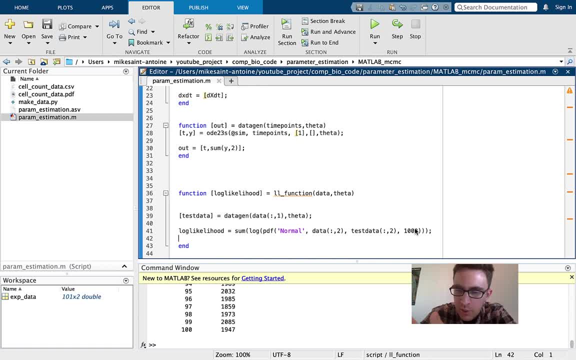 As long as this actually works and we get the correct parameters that actually were used to generate the data, then it's okay to be taking these shortcuts. But again, if you're, if you're trying to write like some kind of like math theory paper, you might want to be like more rigorous about like choosing the actual, like proper distribution and like proper standard deviation and stuff like that. 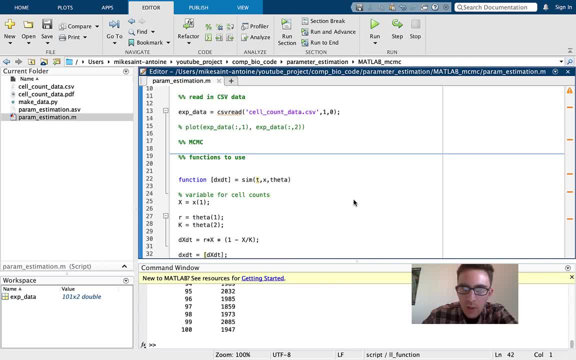 Um, okay, so we're gonna be using, like, all three of these functions to actually to actually write this Markov chain Monte Carlo method. So, again, we're going to be using, like all three of these functions to actually to actually write this Markov chain Monte Carlo method. 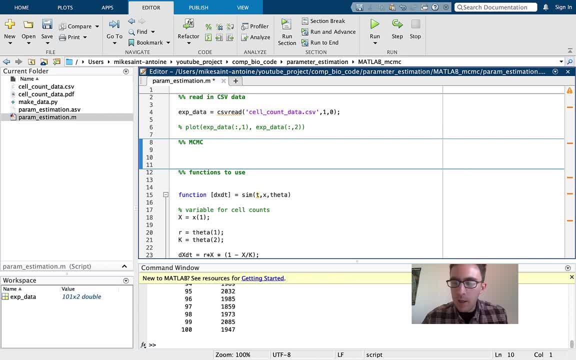 And this is basically a way of like exploring around the parameter space that is going to choose parameter guesses from some prior distribution of the parameters that we, that we set is basically going to be like like evaluating this log likelihood score at a bunch of different guesses and trying to generate some kind of like posterior distribution based on, based on some like maximization of these log likelihood scores. 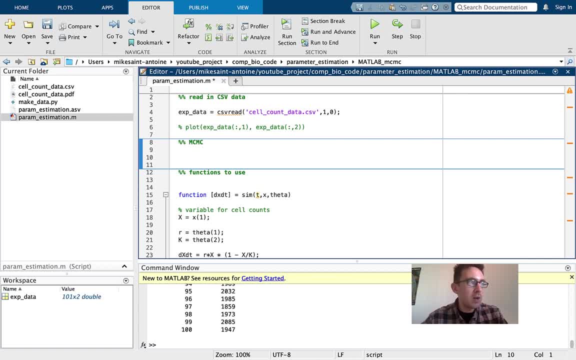 Um, okay, so let's try to actually like get into writing this MCMC method now. So the first thing we're gonna do is just come up with the first guess for the parameters. So I'm just gonna make a comment here: just call this first guess for params. 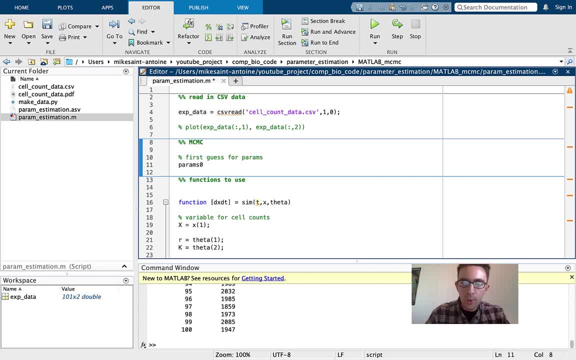 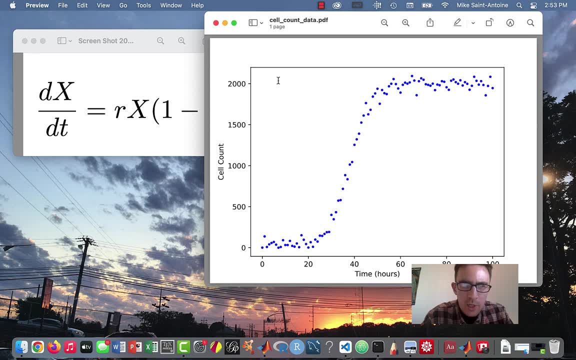 I'm just gonna call it maybe, sorry- params, params zero, just like the first guess for the params. Again, we could kind of cheat, we could like look at the data and kind of already make a guess for what the carrying capacity is. 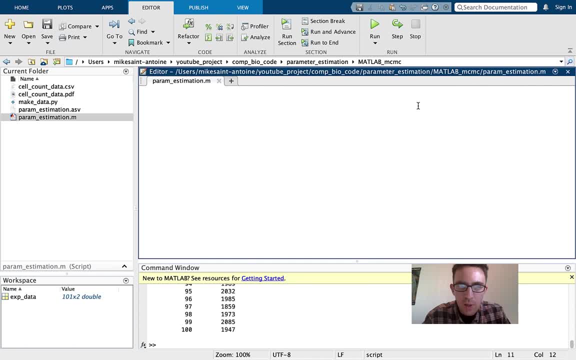 But let's not, Let's not take the easy way out. Let's, let's try to actually like give this algorithm a bit of a challenge and not just take the obvious guess. So let's actually- um, let's just guess one for the growth rate. 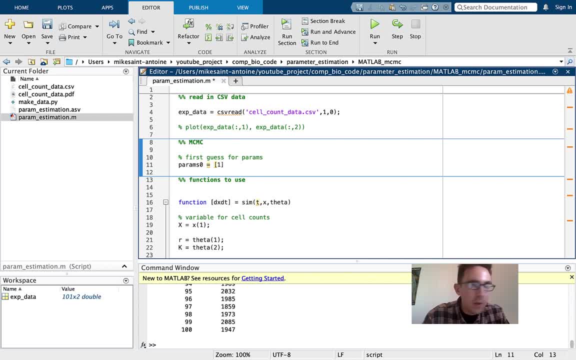 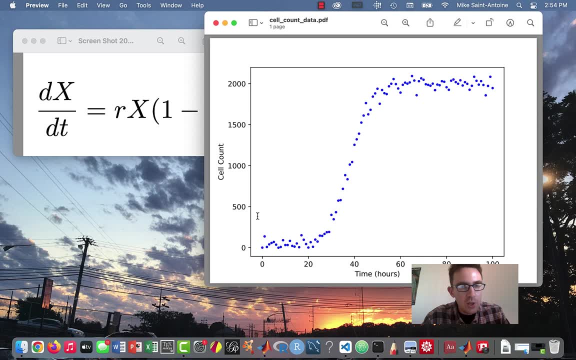 The growth rate are. we'll just guess one- Sorry, uh, semicolon here- And then we'll guess 100 for the carrying capacity. Again, yeah, we can see that realistically it's not going to be 100. But I'm just kind of throwing in the guess that I already know is kind of wrong. 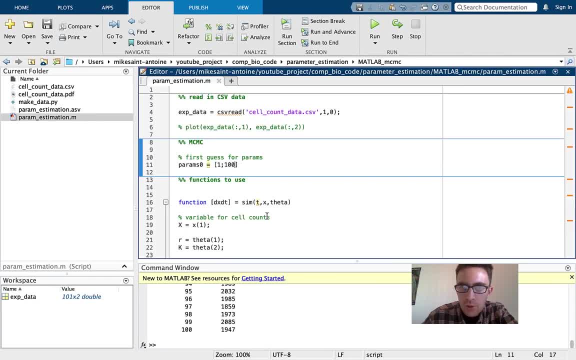 Just because I want you. It has to see that the algorithm can actually get it right. Even if our first guess is is not actually correct, it will actually like solve for the correct value. Um, okay, So then, based on this first parameter guess, we're going to compute a first log likelihood score. 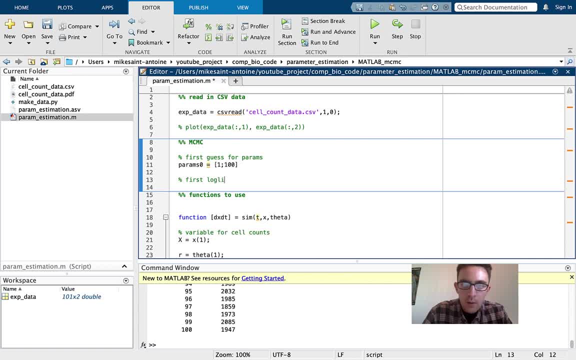 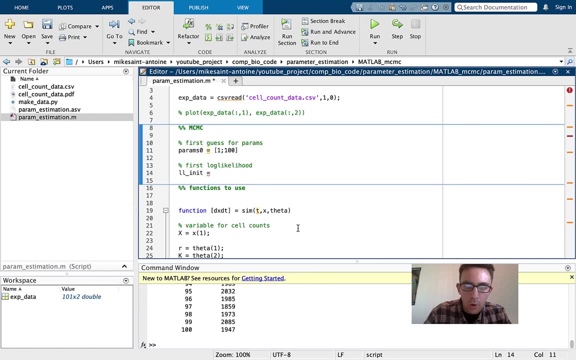 So um log likelihood, first log likelihood. I'll call this: ll init Um equals, uh, what I call this again. Oh, yeah, ll function. Sorry, I forget what I call things here. ll function, um, we're going to pass in our experimental data. 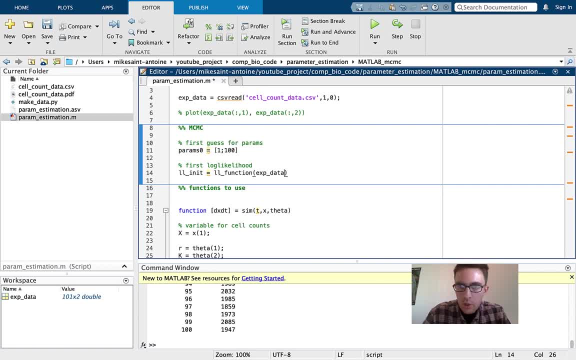 Remember that we write in from the CSV: whoops, experimental data. uh, pass that in for the first argument and then pass in the params um. our first guess for the params Um. oh yeah, sorry, I keep forgetting. you need a Matlab. 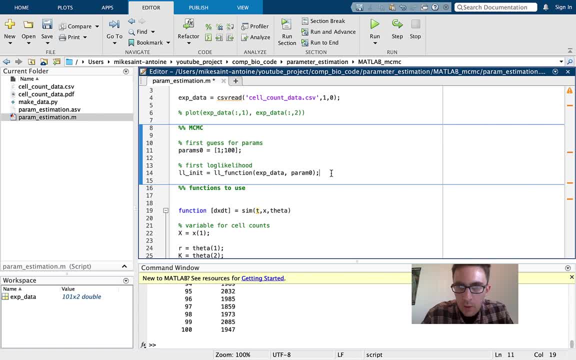 You need to. you need this. I'm going to use semicolons, otherwise it'll just um print all these lines. Yeah, I get, I get spoiled using Python. I'm not used to like writing these semicolons at the end of the lines. but yeah, Matlab, I guess you, you kind of have to do it, or otherwise they'll just print everything. 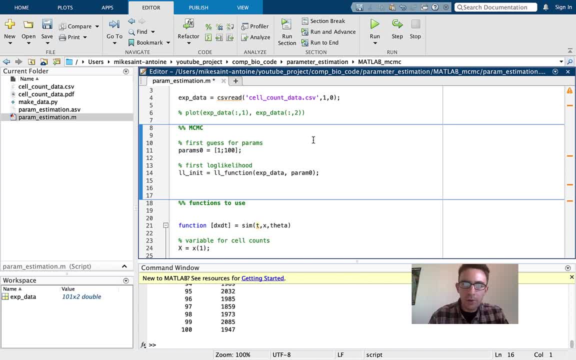 Um, okay, So we have our first guess for the params, first guess for the log likelihood, And then basically what we want to do next is we want to define some arrays to like keep track of everything. So I'm just going to say for comment: um, keeping track of params. 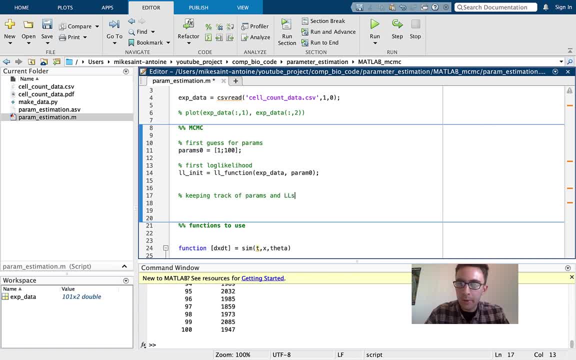 Okay, Params and um log likelihoods. Um, so I'm just going to call this like para set. for the params set, It's going to be some like empty array here And then, um, we're basically just going to like: this is just some fancy notation, but we're basically just going to be appending to the uh, para set. 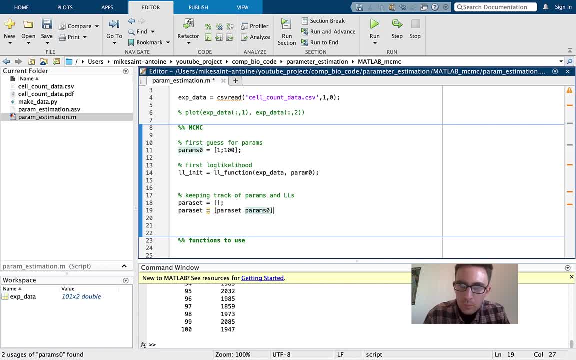 It's going to be appending our first guess for the params. So, yeah, this is just defining some like empty array Here, And then this, this line is basically just appending. appending this param guess to the para set, Um, yeah, basically just just adding it onto this array. 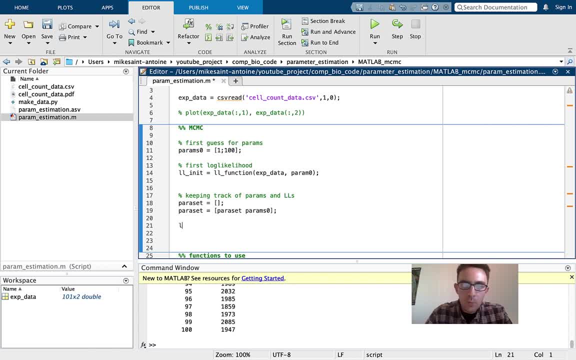 Um, that's just kind of the notation for that Um. and then we're going to do the same thing for the uh, for the like, the log likelihood, um, log likelihood, uh, all of our log likelihoods. 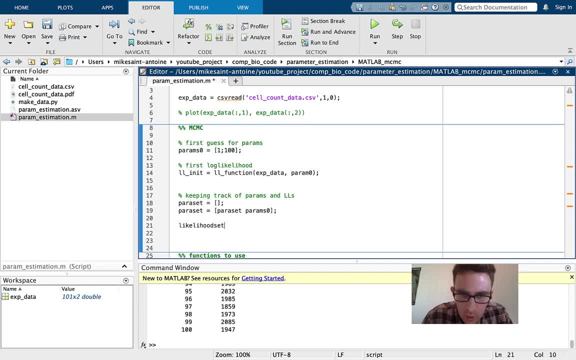 I'm just going to call this the uh likelihood set, Actually, Maybe, yeah, maybe. just to be precise, I'll just call it, um, called the log likelihood set. Um, yeah, just start this off as a uh empty array. 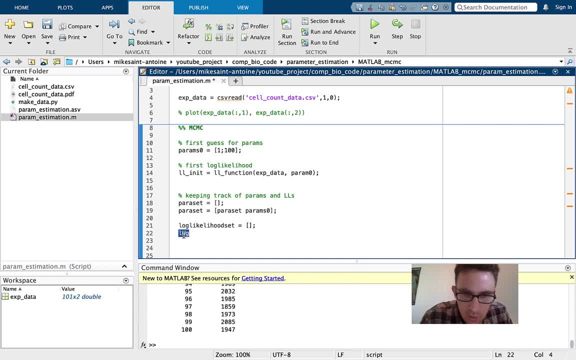 Um, and then you know, just copy and paste this log likelihood set. uh equals um. it's going to be appending our initialized uh first log likelihood. Yeah, Again, just don't get too confused about the notation here. 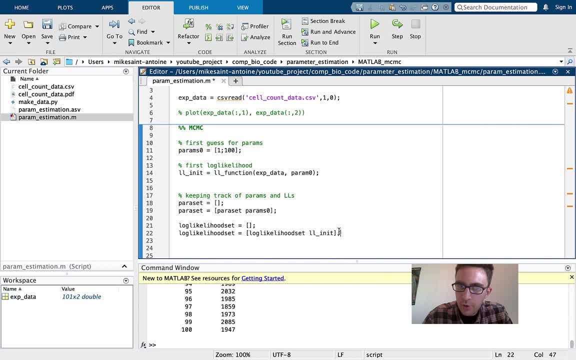 This is just appending. This is just appending our first log likelihood Log, likelihood Log, likelihood to this um log likelihood. uh uh, empty array that we have And then. so the last thing to keep track of is going to be: um, all of the guesses. 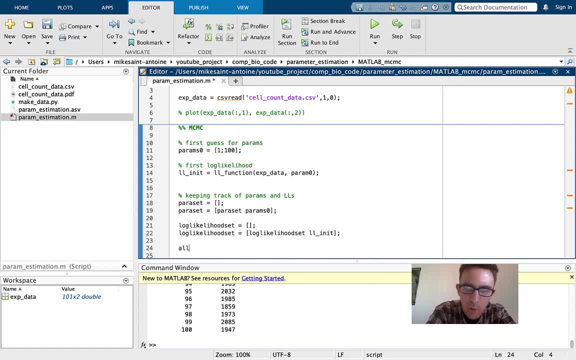 Uh, because basically the way this algorithm is going to work is that some of our parameter guesses we're going to accept and save, And then some of them we're going to reject. But even the ones we reject, we want to still keep track of them. 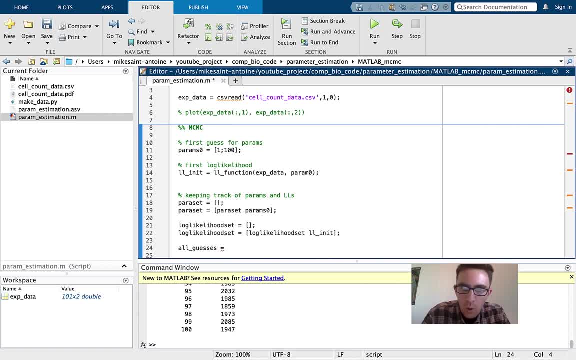 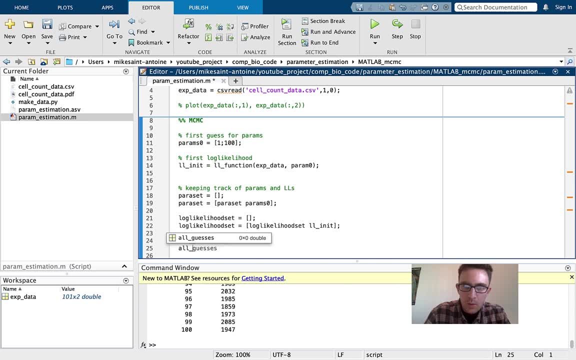 So we're just going to have some, uh, empty array called all guesses. It's going to keep track of, like, all the parameter guesses, whether we accept them Or reject them, since we'll say all guess is again same notation here. 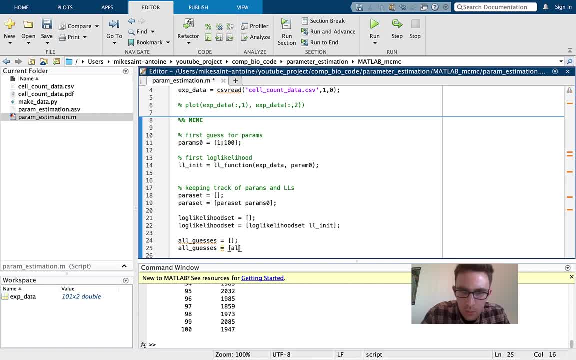 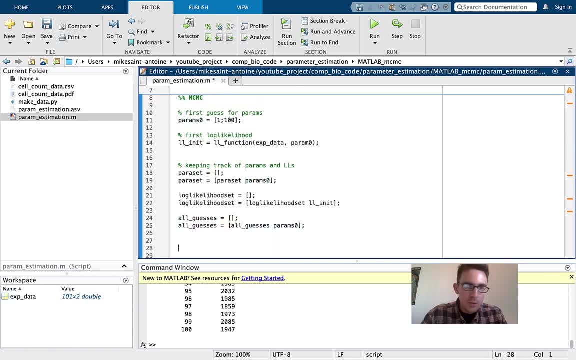 We're just appending, um, we're just appending our first parameter. guess, Um, yeah, Okay. So yeah, these are just like three, three arrays to keep track of things. We're going to be keeping track of the parameters that we accept. 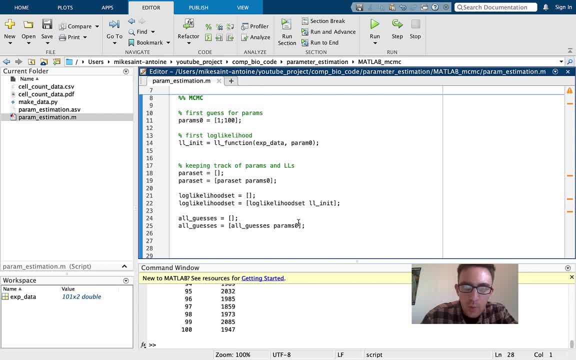 We're going to be keeping track of their log likelihood scores and we're gonna be keeping track of, like, all of the parameter guesses, even the ones that we reject. Um, okay, so now we just need to like- we're going to be basically just like doing a bunch of random guesses and we're going to put all of this inside of a for loop. 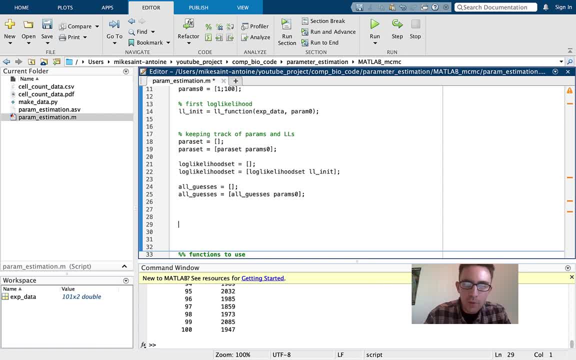 So we just need to set some, some amount of times. we want the for loop to um run. So I'm just going to call this like run Whoops, Sorry, Run uh num, Just the number of times we're running it. 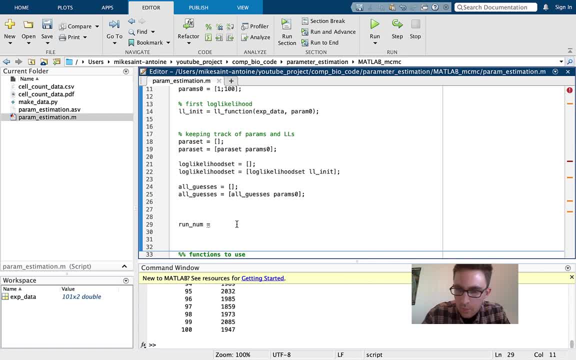 I'll just make this like a million for now. You guys could make it like more or less, uh, depending on, like in a real life situation You'd probably want to have it be kind of a lot, like maybe even more than a million. but for now just make it a million, just so that we can uh get to run kind of test things out. 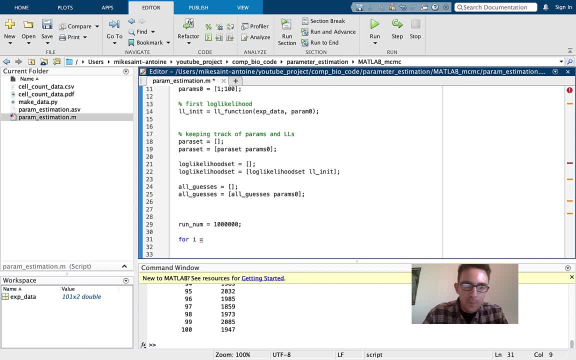 And then we're going to say: for I equals, I equals the range two to our uh run num. And we're starting at two because, like the first one we already just kind of did out here, Like our, our first parameter guess and our first log likelihood score, we already just just did. 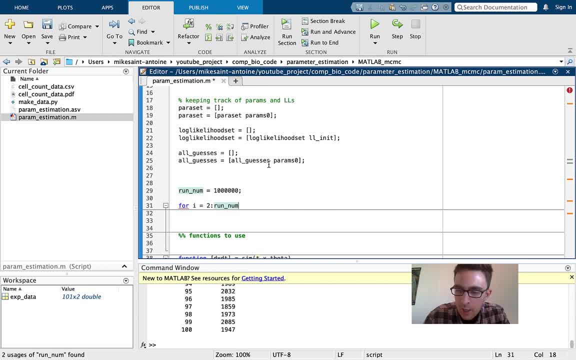 So we're starting with actually the second. the second guess That's where we're starting with two here and then going up to the range um run num. It's going to end this for loop And then something I like to do when I'm doing these like huge for loops is I like to just keep track of the progress. 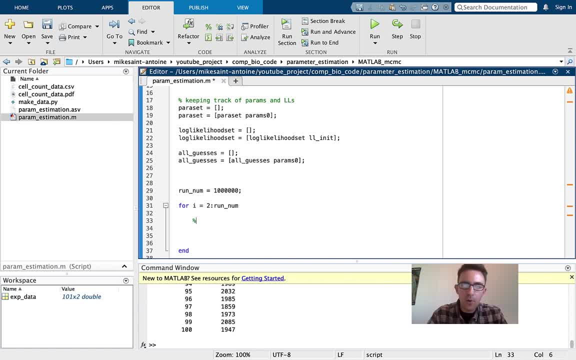 So I'm going to just put in something here: Just keep track of the progress, Um and like see what percent completed is while it's running. uh, keep track of progress. So I'm going to say if, if the 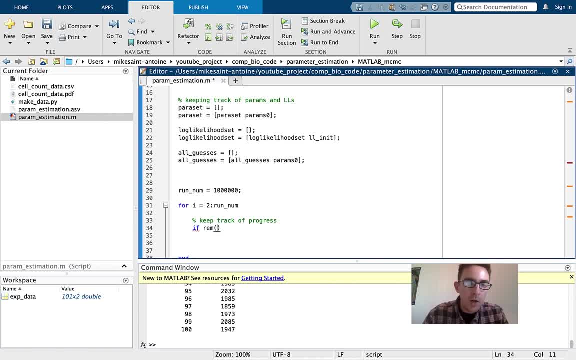 If the division remainder, just rem here. that's just the remainder. when you do a division, when we divide i by 100, if this is equal to zero, remember to end this. So if we divide i by 100 and the remainder is zero, 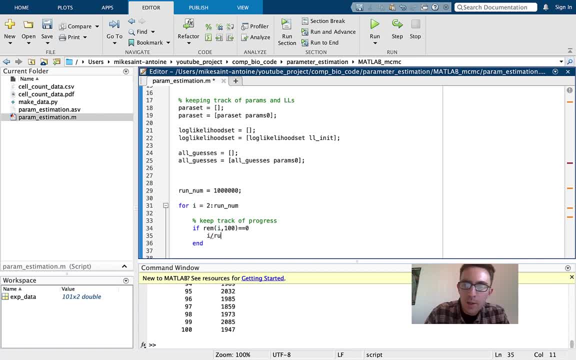 we're just going to print i divided by random, And so basically every hundredth iteration, this is just gonna print out what percentage complete we are, And you guys don't even need this. you guys could just ignore this or whatever. just skip over it. 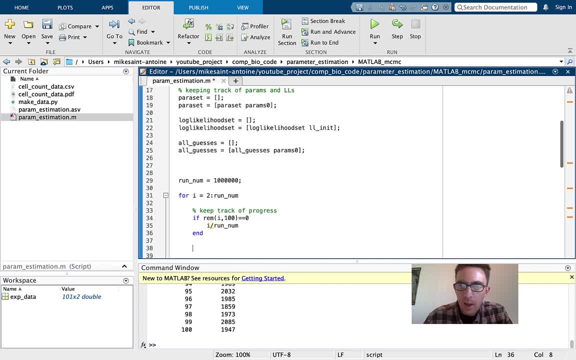 But this is just gonna allow us to see the progress and how quickly our for loop is running. So while we're running- because it might take kind of a long time- we wanna make sure it's making progress and kind of getting things done. 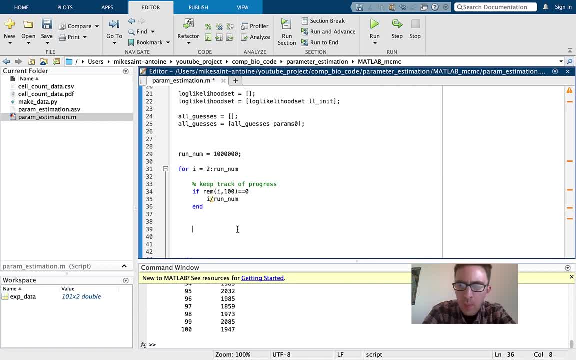 Okay, so now for each one of these iterations we want to guess a new parameter set to try out. So basically we're just gonna say: param test equals. I'm just gonna make this array to store, like both of these parameters here. And now for our guess for R. 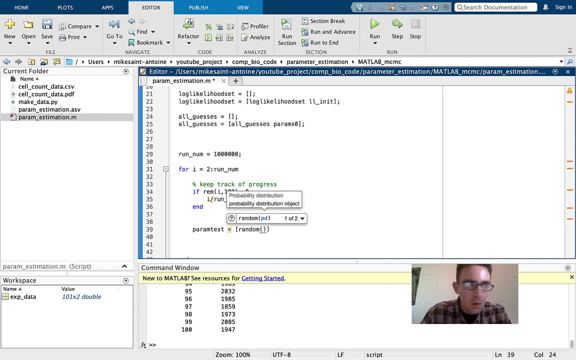 we're just gonna say it's gonna be a random uniform distribution ranging from, let's just say, zero to two. Basically, this is gonna be our guess for the, the growth rate R. Again, this is the great thing about MCMC. 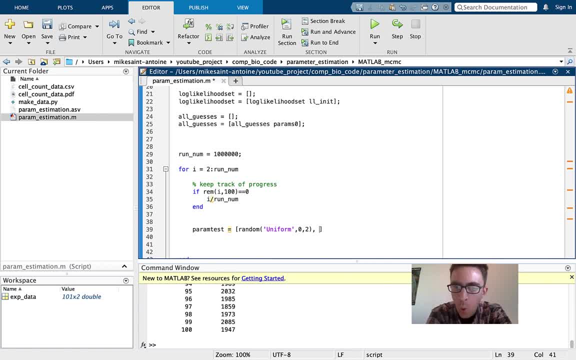 is that you guys can actually make it whatever prior distribution you want to. So if you had some guess about what you thought the growth rate might be, you could make this like. instead of just a uniform distribution, you could make it like a normal distribution. 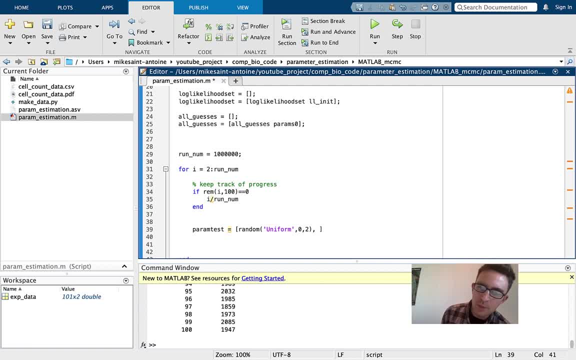 around some guess that you have or any kind of other distribution. But I'm gonna say for now that we don't really have any information, except that we're guessing that it's some value between zero and two. But we're just gonna say between zero and two. 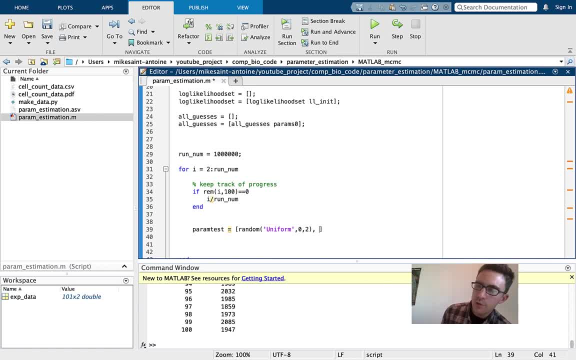 all of those values are equally likely. So our prior is just a uniform distribution between zero and two. But again in a real life context you guys might have like a better guess that you could make like some kind of actual, like normal distribution or something. 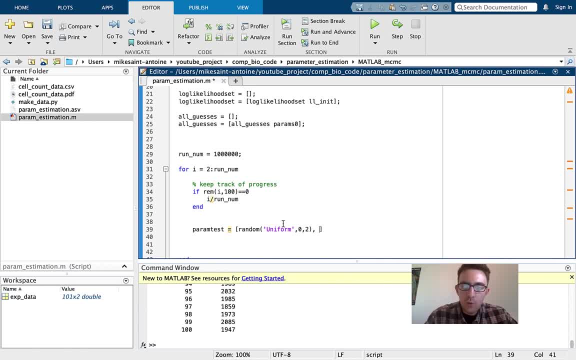 around some guess that you have. But yeah, so this is gonna be our guess for R. And then, oh whoops, I need to actually semicolon rather than comma here. And then for for R, for our carrying capacity parameter. 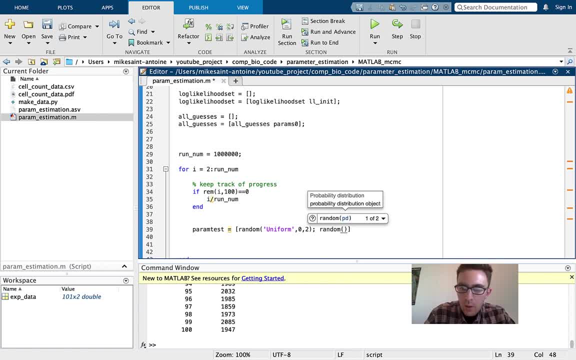 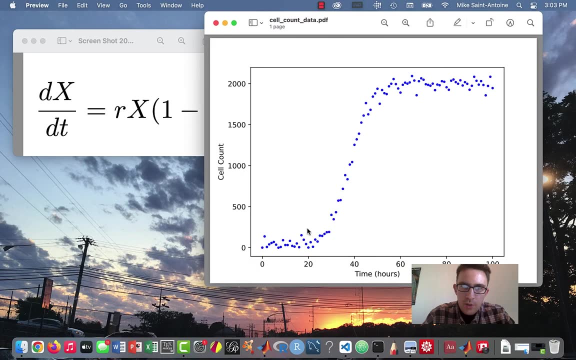 our guess is gonna be a random distribution- I mean sorry, random, sorry, not normal uniform distribution ranging from zero to 10,000.. Again, I'm just trying to show you guys that, even though we can kind of see what it is visually, 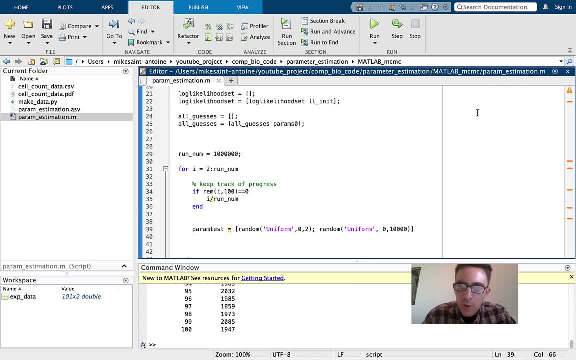 I'm trying to show you guys that even if we like don't take the easy way out, we can actually. we can actually like have this method work. even if we don't tell it what the correct carrying capacity is, We can have it actually get there by itself. 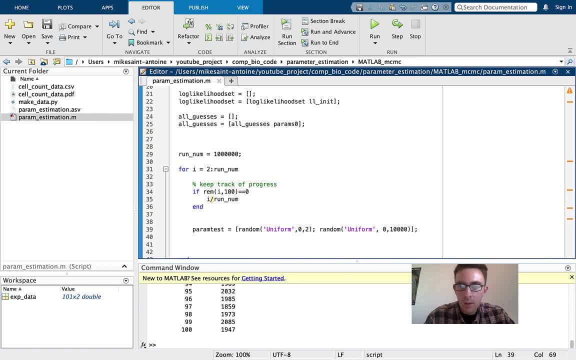 just by the method actually working. Okay, so for each iteration, this is our guess for the parameters. You guys may also see different methods of doing the guesses differently. For example, you may see another method called gib sampling, where you change the parameter guesses. 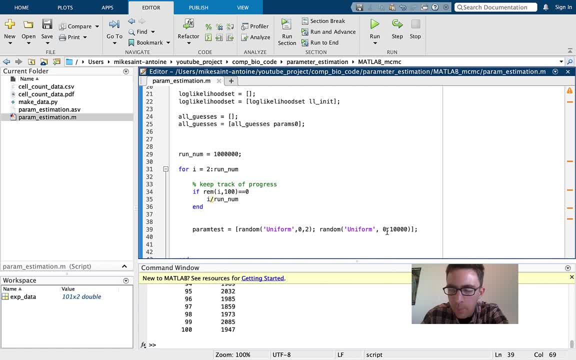 guesses like one at a time, like for each one, instead of changing both of them. you keep the previous guess for one of them and change the other. um, that's something called, uh, called gib sampling, but for now i'm just kind of like kind of making this as simple as possible, just for each. 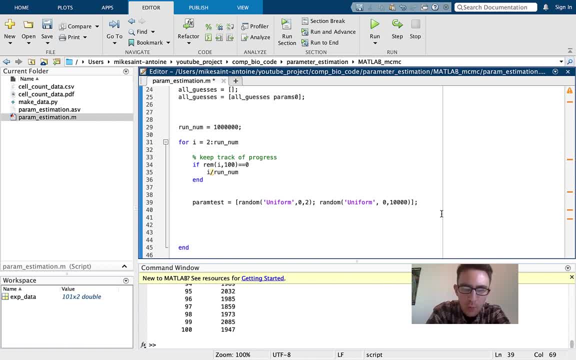 one. generate um. generate a new like random guess for both of them. okay, and then for this, for this guess of the parameter set, we're going to um generate um. generate the log likelihood school for it. so we're going to call this log likelihood um. ll test equals ll function. um passing in the. 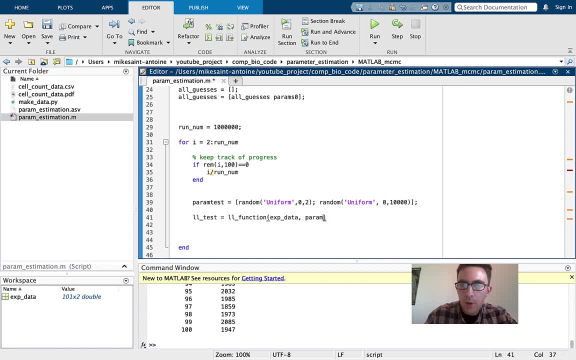 experimental data and uh- our test parameters. it's called param test here. so again, this is just generating like a uh, like a new parameter set guess and then the log likelihood score for this guess. so now what we need to do is this thing: um, i'm going to do this thing called the uh metropolis. 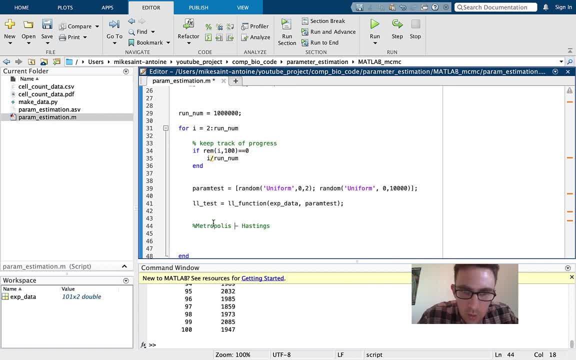 uh, hastings algorithm. uh, the idea with the metropolis hastings algorithm is basically that if, if our um, if our log likelihood score is better than the most recent saved log likelihood score that we have, if it's better than that last saved score, we're going to um definitely accept this. 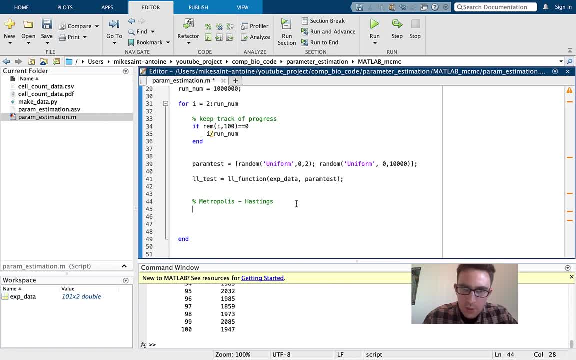 parameter set and save it. uh, but even if it's, even if it's worse, we're going to, um, we're going to basically like roll the dice and and give it some like random probability of still being saved anyway, just so that we can, um kind of keep exploring around the parameter space and sort. 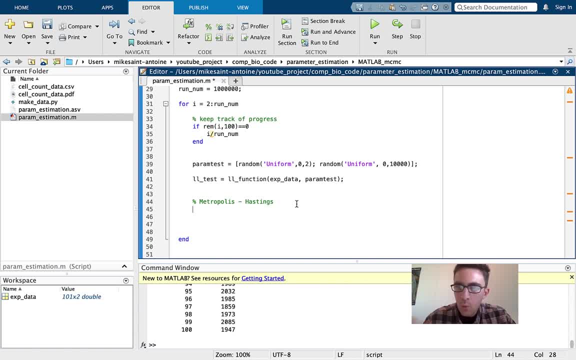 of keeping some level of uncertainty um within our uh choice of um which parameters we're accepting. we're incorporating some uncertainty uh into that even so, basically, if, if the log likelihood score is is better than the most recent saved one, we definitely, we definitely save these new parameters. 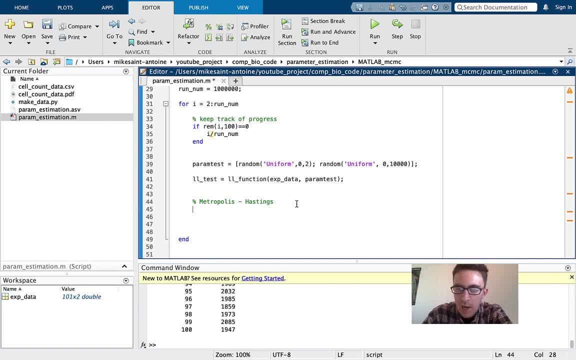 but even if it's worse, then we still, with some random chance, we still may end up saving it. and the way we're going to actually implement this is we're going to say: if ll test equals- sorry, not equals um- if it's uh, greater than or equal to um, the whoops log. 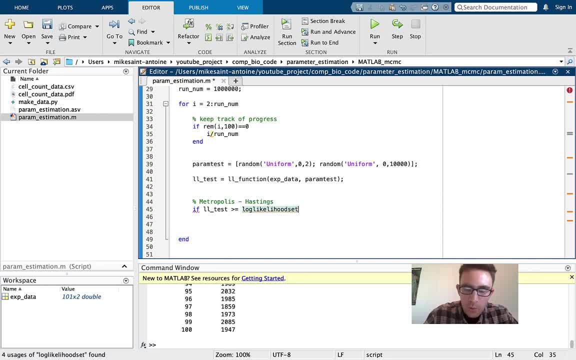 likelihood set. remember, this is where we're saving all of our um, accepted lovely counter likelihoods, all these log likelihood scores. We're just going to get out of this the most recent element that we saved. So, basically, if we just left the if statement like this, basically this would: 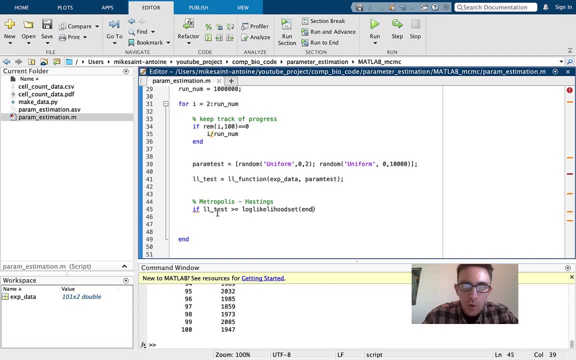 evaluate as true if our most recent log likelihood score was as good or better than our most recent saved log likelihood. but we wanted to, with some probability, still accept the parameters, even if the new log likelihood score isn't as good. So we're going to add a term to this and basically say plus and. 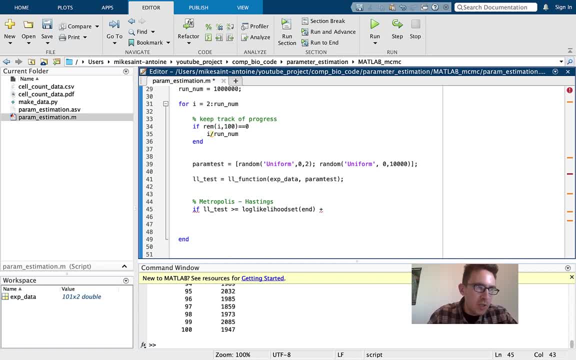 again, it's going to be a bit of confusing math here, but we're going to say: plus log, the natural log of a random random value of the value of a random value of a random value, uniform distribution between 0 and 1.. So basically this is saying we just 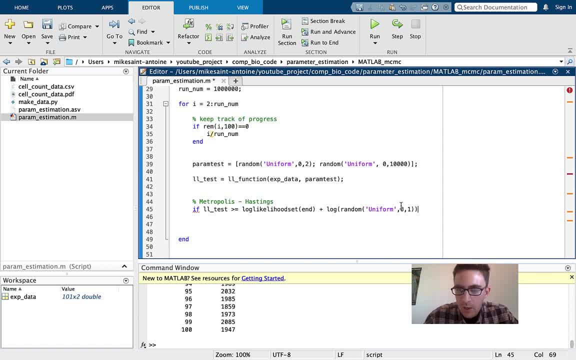 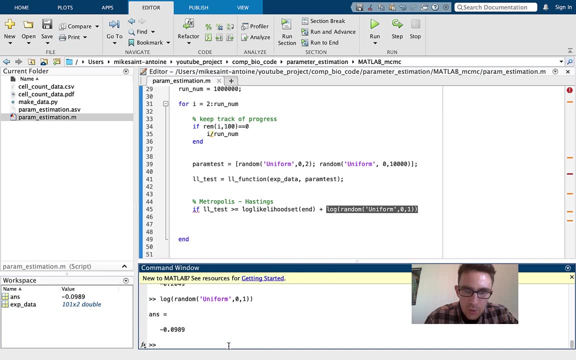 take a random number between 0 and 1 and then take the natural log of it and so basically, this is going to give us some negative number. and just so you guys believe me, I'll just actually like evaluate this, evaluate a couple times here. It's basically giving us like some random number. so 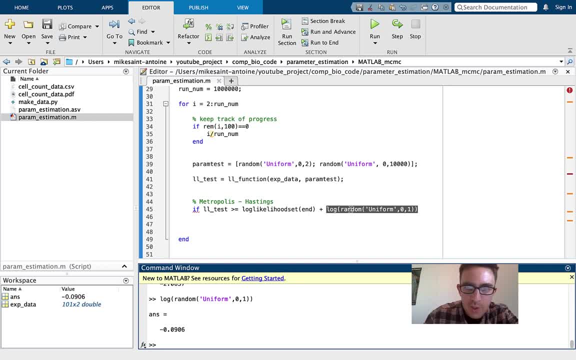 basically this: even though we have a plus, this is going to be decreasing this saved log likelihood score by some amount, some random amount that we're choosing. We're going to decrease this like most recent saved log likelihood score. So we're basically going to be like, by some random amount we're going. 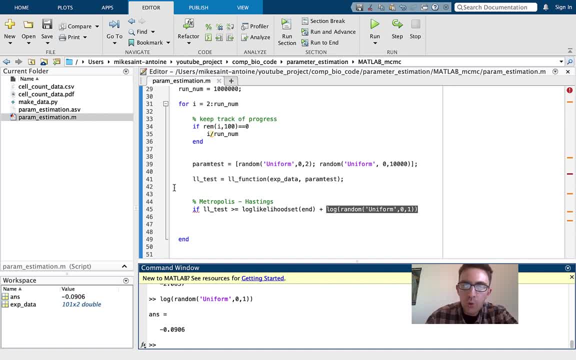 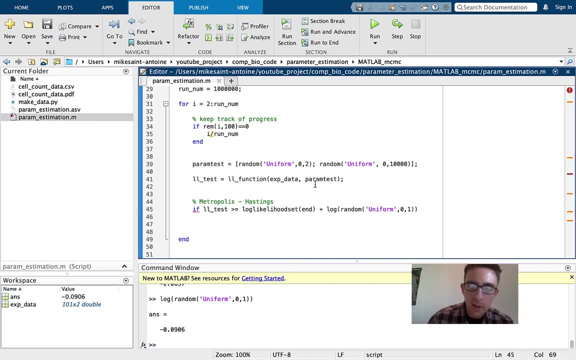 to be like lowering the bar that this new log likelihood score has to meet in order for these parameters to get saved. So, basically, even if the new log likelihood score isn't as good as our most recent saved log likelihood score, there's going to be some like. 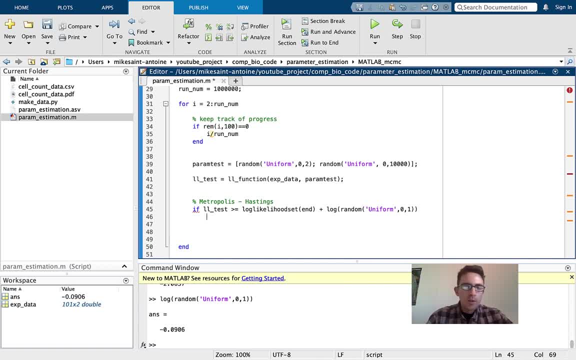 probability that we're still going to accept the parameters anyway. So, basically, if this evaluates as true, we're going to say: we're going to say log likelihood set equals log likelihood set and we're going to append the the new score that we have here, Basically just appending this. 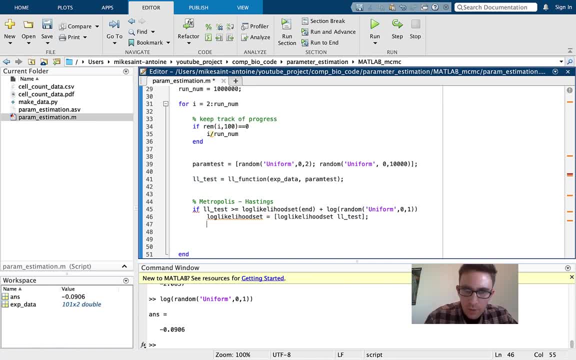 new log likelihood score. Sorry I can't talk, but log likelihood score set that we're saving here. We're going to do the same thing for the parameter set that we're keeping track of. sorry, paris set equals paris set appending parameters test, And then just doing the same thing for all guesses. all guesses two. So yeah, 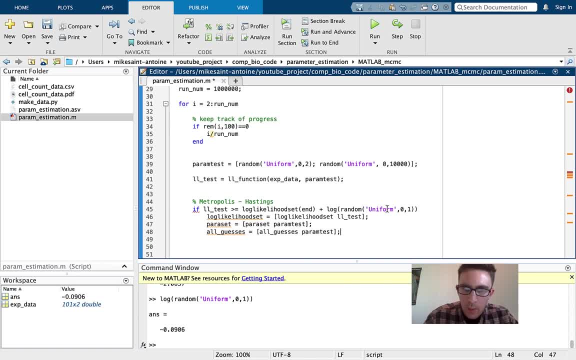 basically, if we're accepting, if we're accepting these, this new parameter set, we save the log likelihood score, we save the parameter set And we also record. we record the parameter set in our like list of all the guesses to remember the. 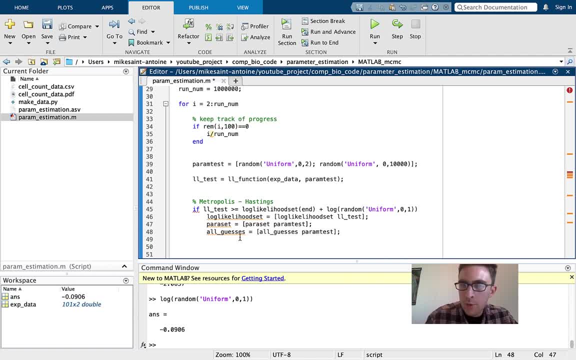 all guesses list is keeping track of even the parameter sets that are going to be rejected. Okay, so what about if we? what about if we? um, if this evaluates to false, then what do we do? So we're gonna say else, basically, in this case, 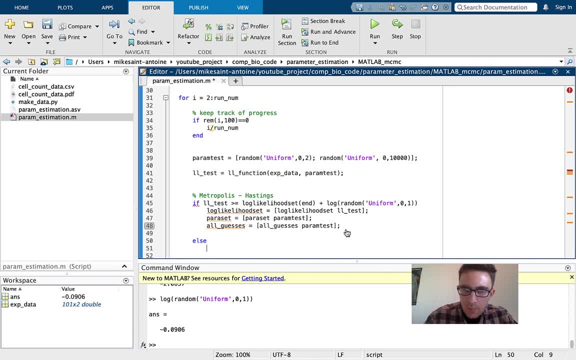 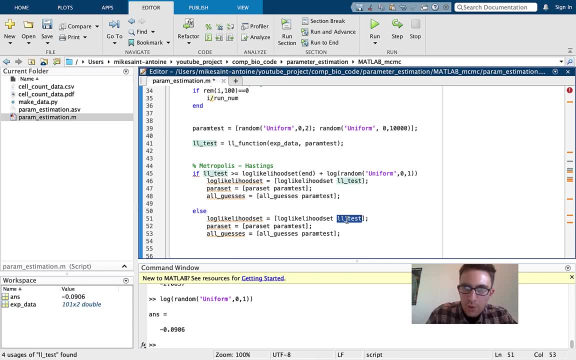 we're going to update all of these again, So I'm actually going to copy and paste this block of code here, But then for these two, instead of saving the new values, it's just going to still save. um, it's gonna still save like the previous. 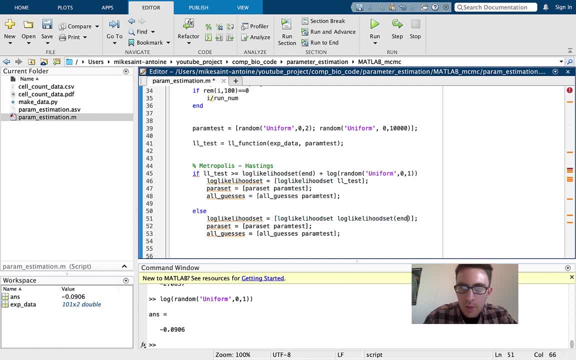 value. basically there's still save this like value at the end. Same thing with the power set Whoops. So basically what we're saying here is that we're not accepting this new value, we're just saving like the previous value that was. 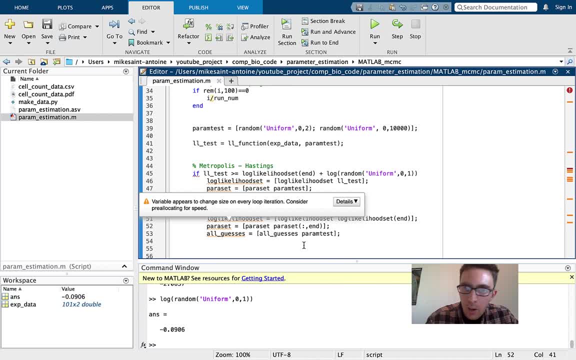 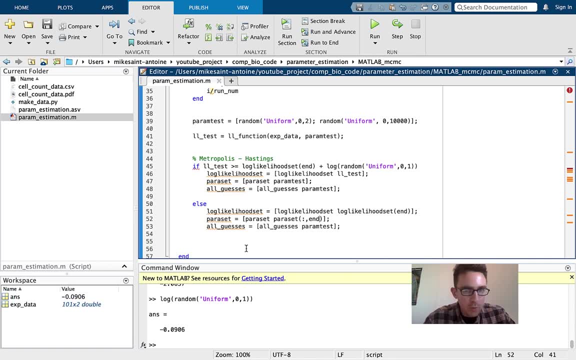 already recorded here which, depending that previous value, um, again, yeah, but then. but then for all guesses, remember all guesses- we want to update this one. even with the rejected um, even with the rejected parameters, we still update to. 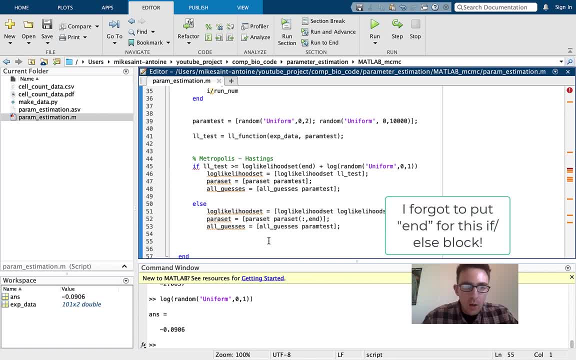 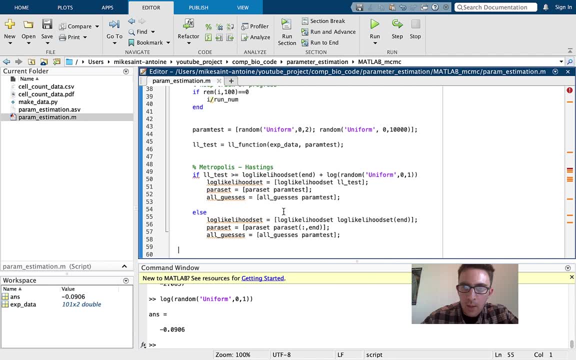 save the rejected parameters into the all guesses. Um, okay, yeah, so this is basically all we need. Um, we're just again iterating through. uh, we're basically just like iterating through this like a million times And each of. 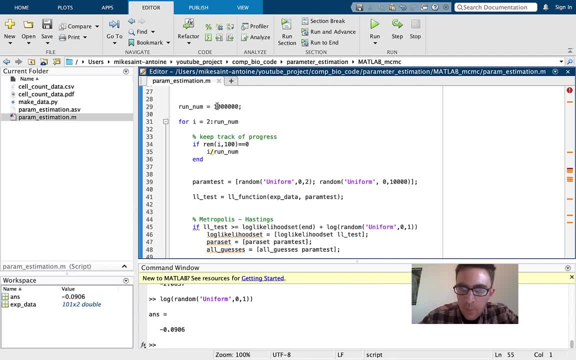 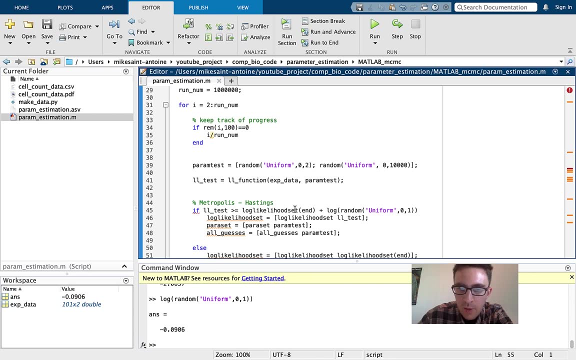 these iterations we're choosing a new guess for the parameter, for the parameter set, and we're computing a log likelihood score for that new parameter guess And then we're seeing how well the log score compares to the previously saved log likelihood score and if it's better. 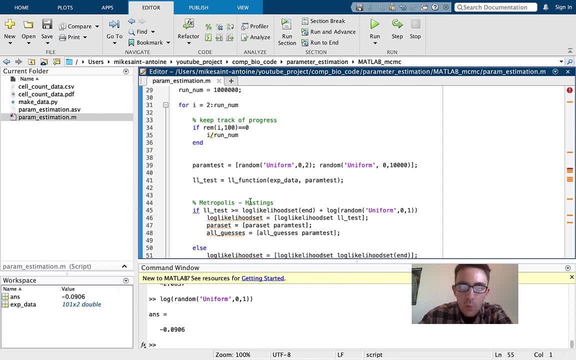 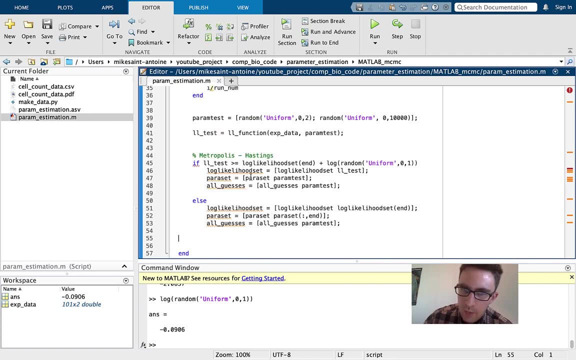 than the previously saved log likelihood score, then we definitely save this new parameter set. but even if it's worse, there's still some probability of it getting saved anyway, just so we can incorporate some uncertainty into like which parameters we're saving, and we we want to save all the guesses, even for. 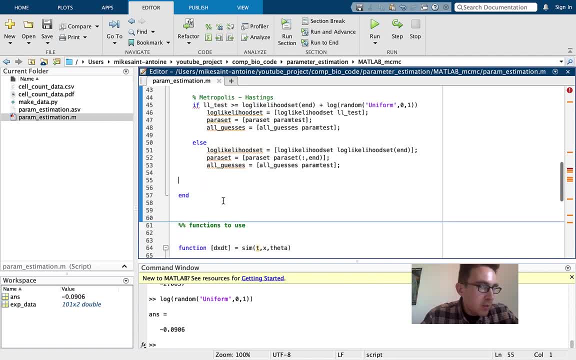 the parameter sets, they're rejected to. Okay, so that's basically it. that's basically all we need for the Markov chain Monte Carlo method, and the last thing we're going to do is actually like plot our posterior distributions to get some idea of like what we're ending up with here for our 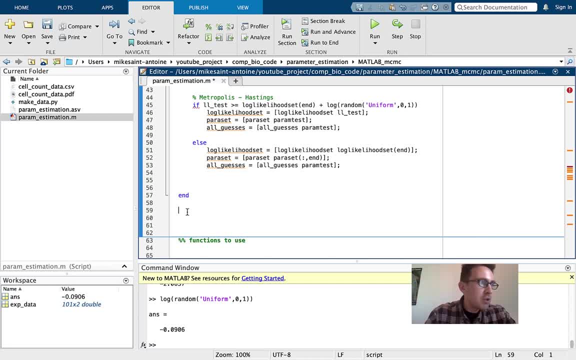 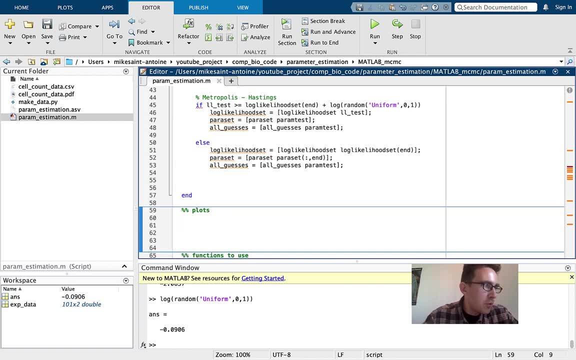 parameter guesses. So it's gonna make some section here called plots and again going to be a little bit lazy here, just going to copy and paste some code in, Just going to copy that in and paste it in. to save a bit of time, I'll kind of explain what the plots are doing. but 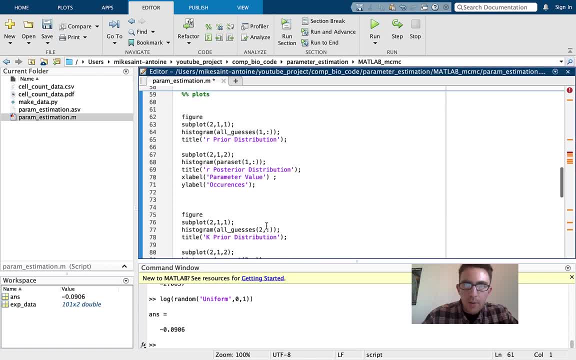 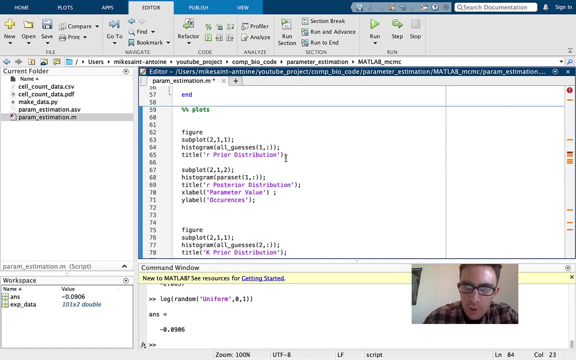 yeah, it's gonna be a little bit lazy here and copy paste some of this in: Yeah, so basically we're just making one figure to plot our, our parameter distribution. so we're gonna plot the prior distribution which, remember, we're saving, since we're saving all of our guesses, they're just being sampled from. 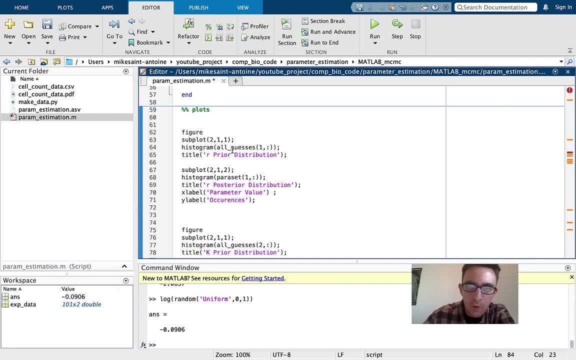 the from the prior distribution. we're really just plotting a histogram of all of our parameter guesses and then we're also plotting a parameter. we're also plotting a distribution of our saved parameters, which is gonna be our posterior distribution, and you guys are gonna see what this ends up looking like. 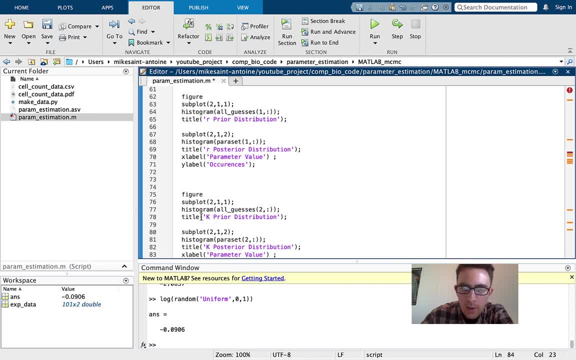 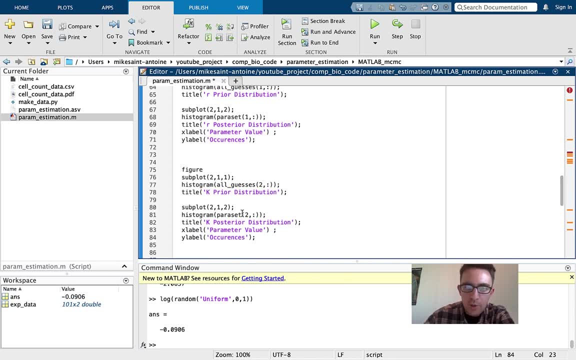 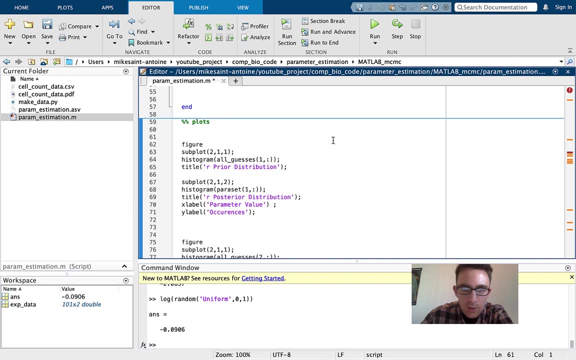 and then we want to do also the same thing for our K carrying capacity parameter. we're just gonna plot on one histogram of our prior distribution and then another histogram of our posterior distribution. Okay, so I'm just going to run this code. hopefully it works. okay, we're gonna see when the plots come out. 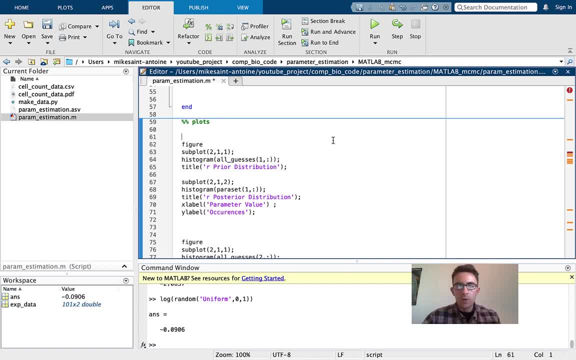 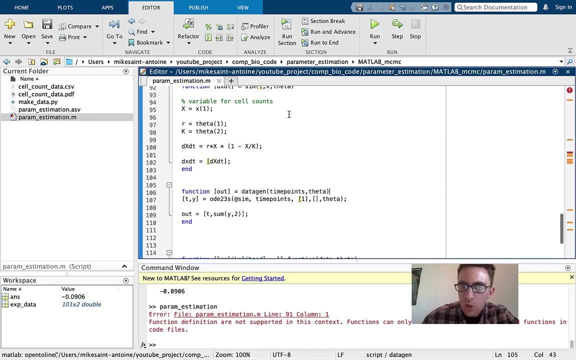 if it, if it hopefully turned out to be okay. so fingers crossed that this actually works. oh, maybe I'll save it first, but okay, yeah, let's give it a shot. okay, wait, okay, we got some some error here. sorry guys, give me like one second to figure out this error here, okay, guys. 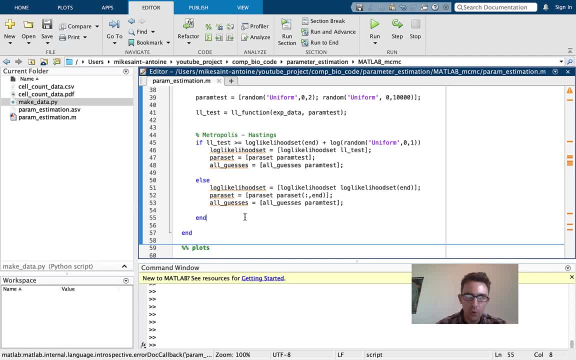 sorry about that. I just had like two bugs I had to fix to get it to work. so the first one was that I just forgot this end statement at the end of this if-else statement. so just um, yeah, I just went back and put this end statement in. 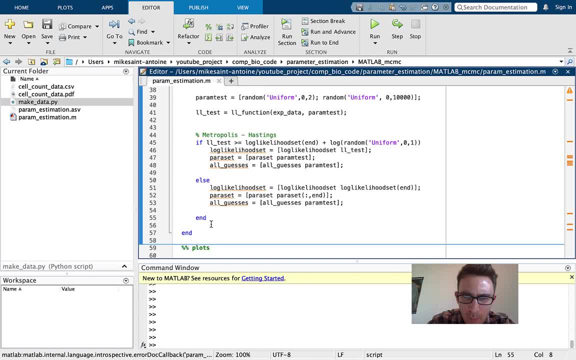 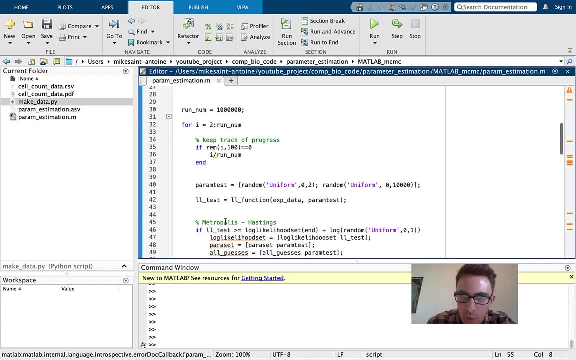 here again. sorry about that clumsy mistake. I'm just not really used to MATLAB, so just kind of get forgetful with that sometimes. but yeah, just added that in. and then I also had a typo that I had to fix up here. so, um, I had put: I 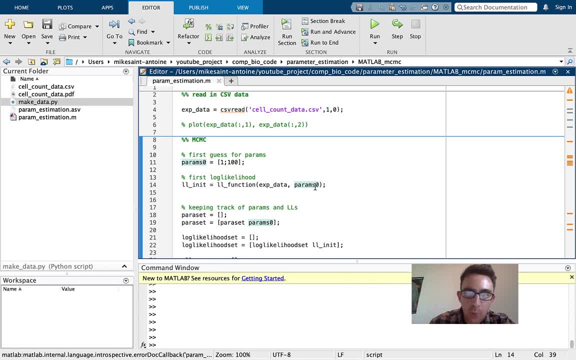 don't know if anyone, if any of you guys caught this, I'll be impressed. but maybe caught it while I was typing it. I put param zero. It should be params with an S, params zero. So I just had to fix that typo there. But yeah, that was the one bug. 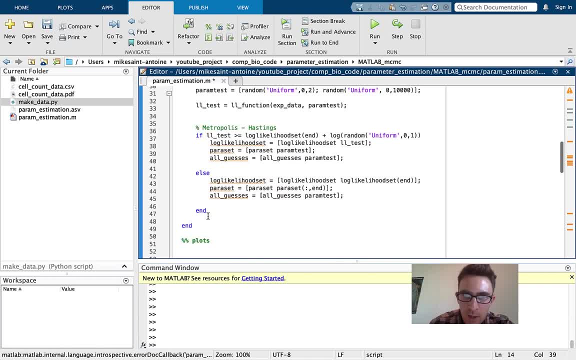 And then the other bug. just this end statement at the end of this, if else. But okay, so I think it should be running fine now. So I'm going to run it and then we'll check out the results. Yeah, so remember, this thing it's printing here is just our progress. 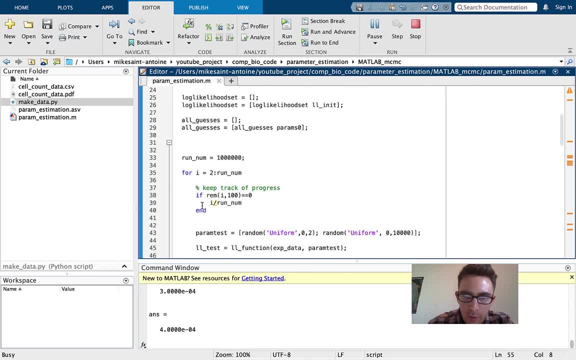 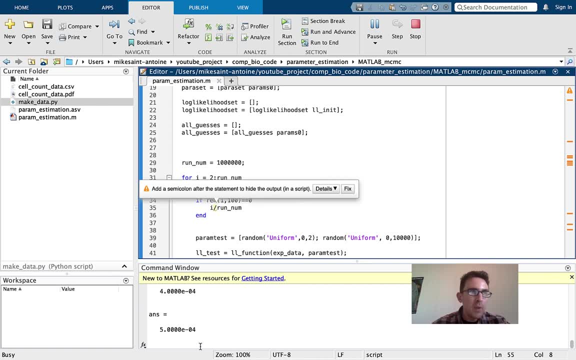 So remember, we printed out basically every hundred iterations. we're printing out like the percent complete it is. You guys can probably see it's going pretty slowly. That's partly because I'm just using. I'm like I'm recording a video of this. 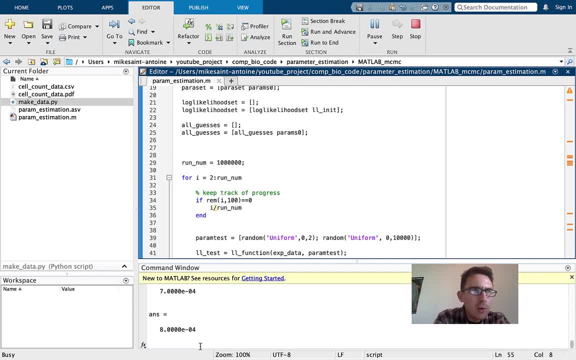 I'm doing like the screen capture video. That's making it go a little bit slower than usual. But even if I wasn't like recording the screen, it would still be going pretty slowly. So at this point I think I'm probably just going to run it. 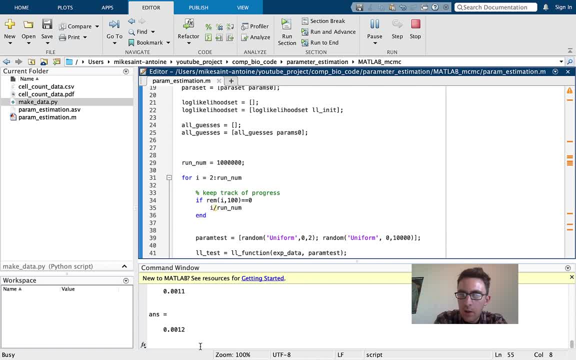 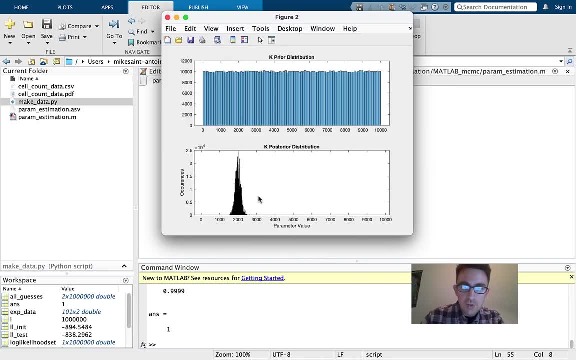 I'm going to cut the video and then I'll just skip towards the end, when it's complete, And then we'll discuss the results. Okay, guys, so now we have a result. You guys probably can't tell on your end, because I cut the video. 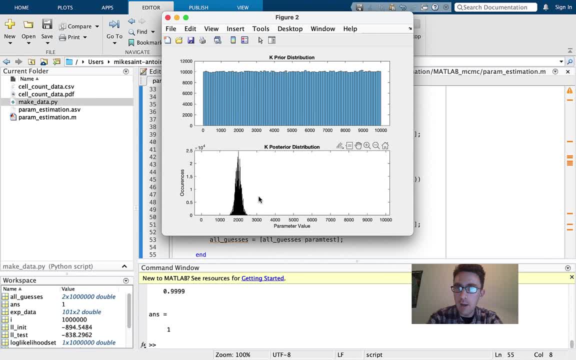 But this actually did take a pretty long time to run. It actually took a couple hours. So I'm going to recommend to you guys as like a general, like best practice: Before you run this thing for like a million iterations, Run it for like a hundred or like a thousand first. 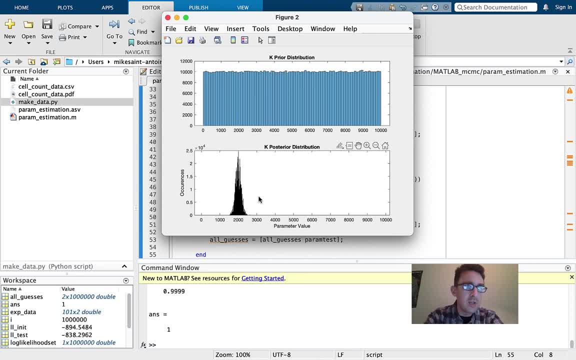 So that you can like check and see if there's any bugs, Because really the worst thing ever in programming is when you have something like that's running, That takes like hours or like days to run, And then at the very end, instead of like outputting a result. 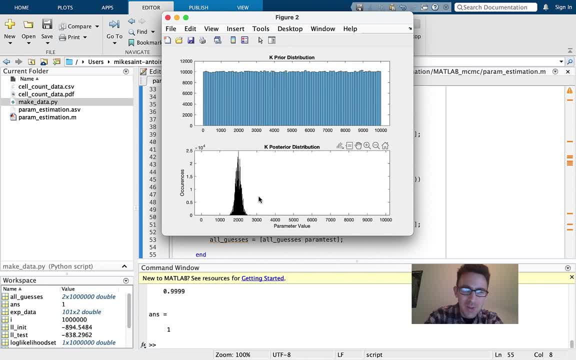 You get some like bug at the end that you didn't realize was going to be there. So, yeah, you don't want to have that happen. So I just recommend to you guys, like, run it for like a hundred iterations first Before going for a million. 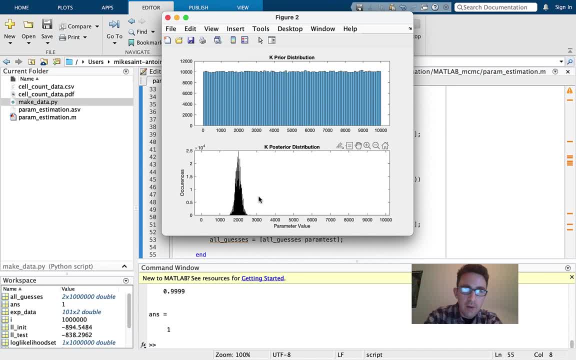 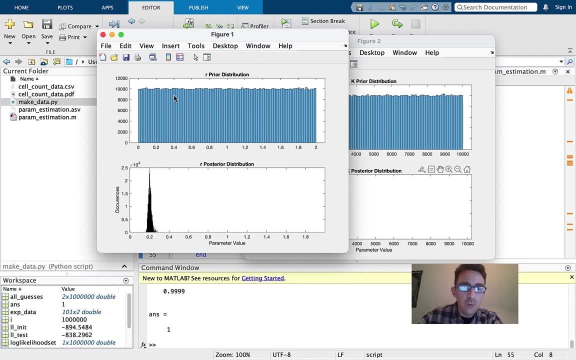 Just to like check and make sure everything's working. But yeah, so now we have a result. So there's actually two figures here So we have. the first figure is our prior and posterior distributions for our R parameter. Remember, R is the growth rate parameter. 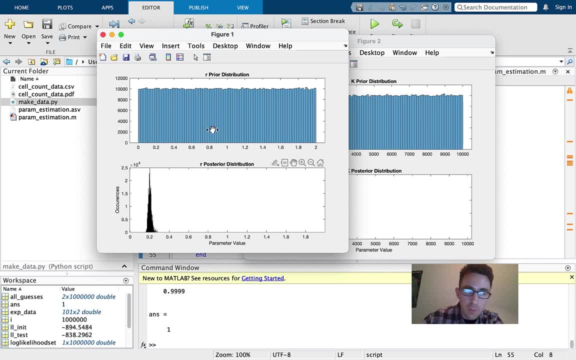 So the prior is what we programmed it to be: Just a uniform distribution between zero and two. Like I said before, if you guys, if you're doing this in a real life context, If you know some like prior information about what you're expecting a parameter to be, 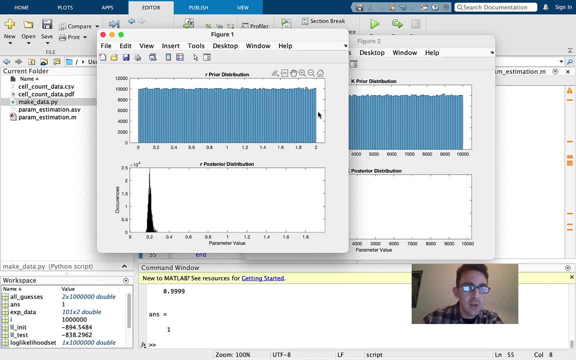 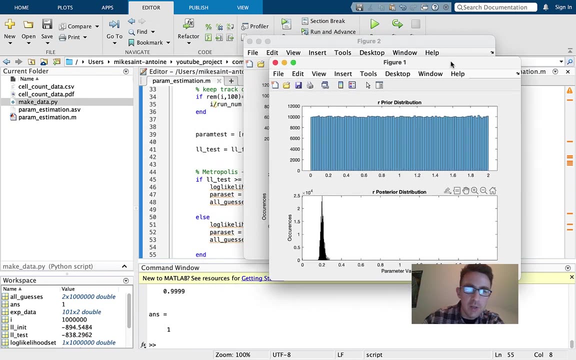 You can make the prior anything you want it to be. You can like include some information about, like what you're expecting. But then our posterior- And remember the posterior- distribution is the distribution of accepted parameter sets That are accepted based on this Metropolis Hastings method. 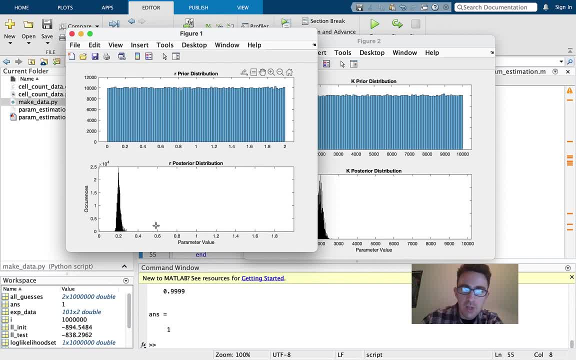 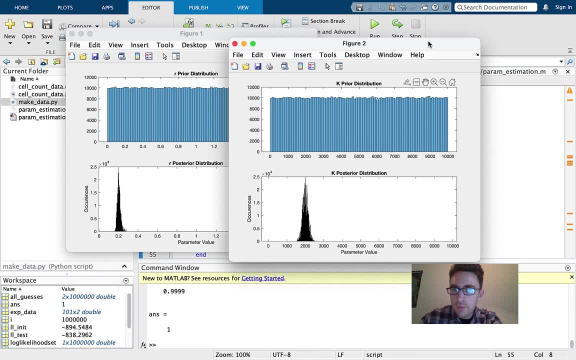 This is our distribution of all of the accepted parameter sets And we can see for the posterior It kind of clusters around 0.2. And then so we have the same thing for our K parameter. Remember, K is the carrying capacity. So our prior distribution is what we programmed it to be. 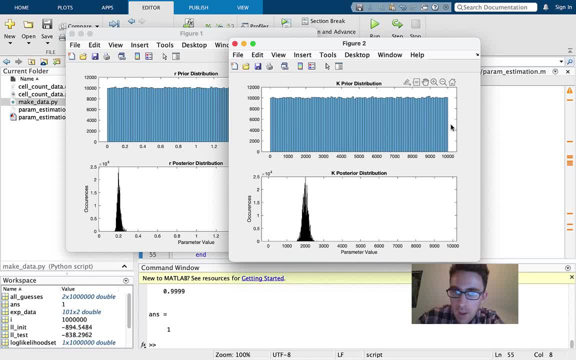 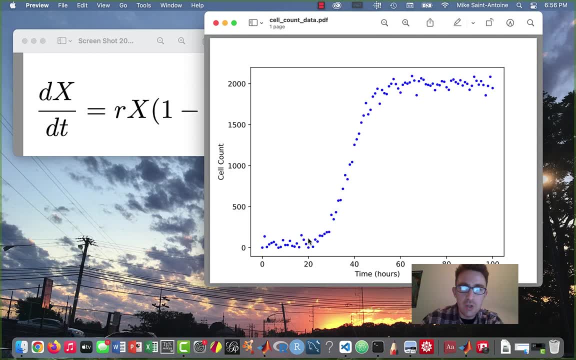 It's a uniform distribution between zero and 10,000.. And our posterior distribution It kind of clusters around 2000.. Which we can kind of already see visually that this is going to be what it is, But we made it Um. 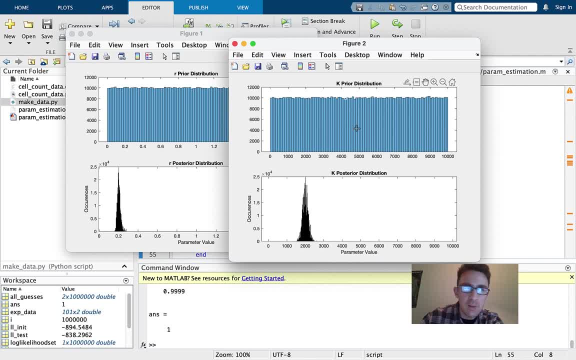 we made it like more difficult than it had to be for the algorithm to like, check and make sure it can actually find the right answer on its own. So we just started with a uniform distribution between zero and 10,000.. And then it looks like it got it right. 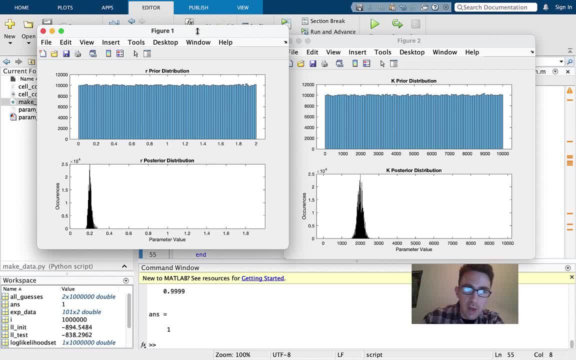 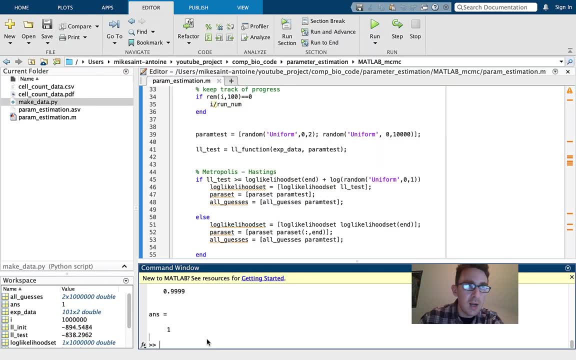 If we wanted to get some like actual numbers out of these distributions, we could actually do things like compute, like confidence intervals. So I'll show you guys. Um, let's just say we wanted to get like the 95% confidence interval for our posterior of our R distribution. 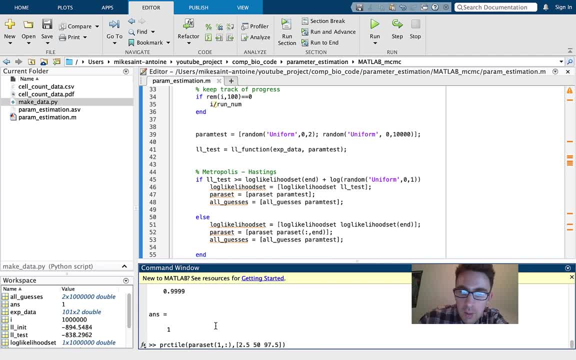 This is how we do that. We'd say like Paraset: Um, we want the uh, the, the first row, which is going to be all of um, all of the uh, all, all of the R values. 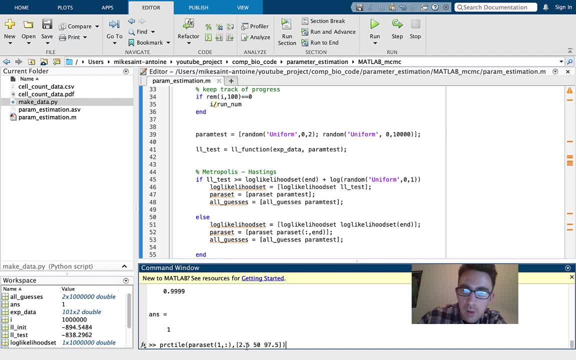 And then we just want the percentile at the 2.5 percentile, the 50th and then the uh 97.5 percentile. This will give us something like a uh, a 95% confidence interval for this posterior distribution. 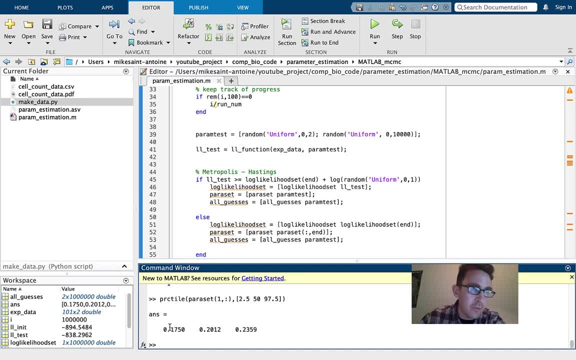 Yeah, And just like we expect it, it kind of centers. It centers around 0.2 and we have we could put like arrow bars on it if we wanted to. we could do the same thing for um, our, our K parameter. 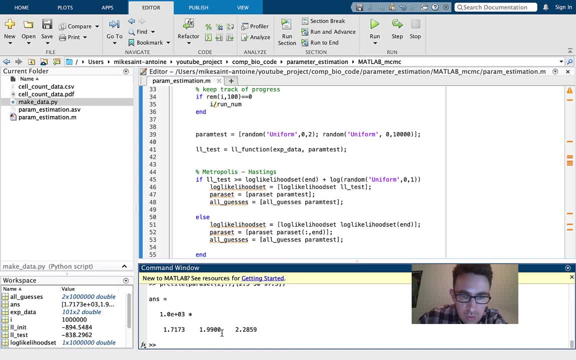 Uh, let's do the same thing there. Um again, it's not exactly 2000, but it centers um, centers around like 1,000, uh, 990.. And I mean, this is, this is like being scaled here. 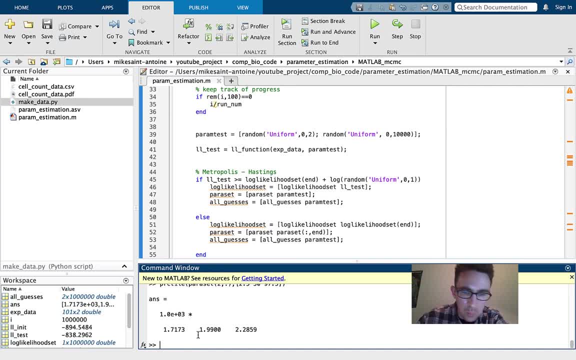 So these are all in the thousands. Uh, so yeah, it kind of centers, centers like pretty close, like 2000.. Um, not exactly, but we could put error bars on on this posterior here. Um, okay, So now for the moment of truth. 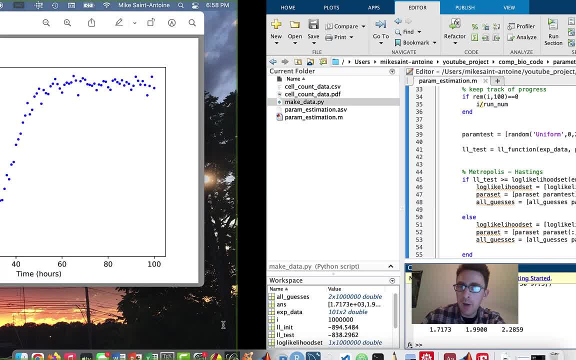 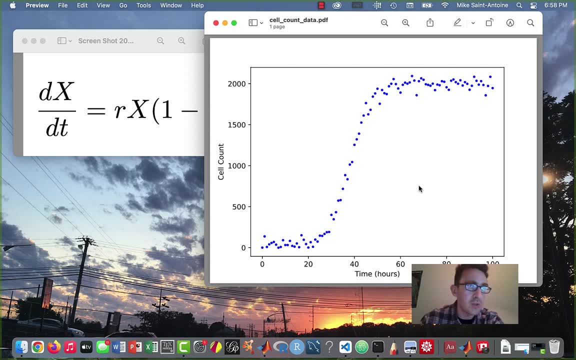 now I'm going to show you guys the code I use to generate this um, this like mock data set, And I'm going to show you guys what values I actually used to generate this like this noisy data set. So here's the code I used in Python to generate the stochastic data. 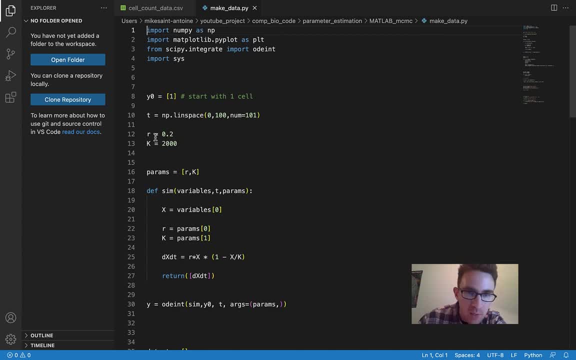 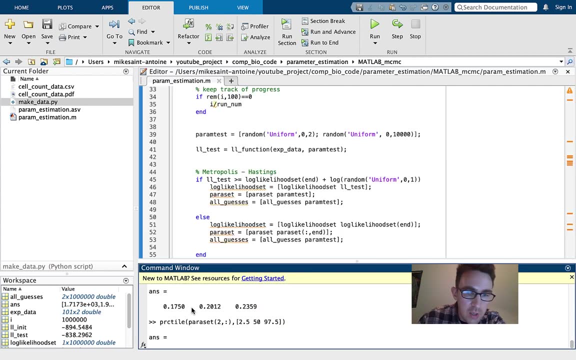 And yeah, so, like you guys are probably expecting, I set R to be 0.2 and K to be 2000.. So we can see that. Yeah, Like our our uh, MCMC um parameter estimation. 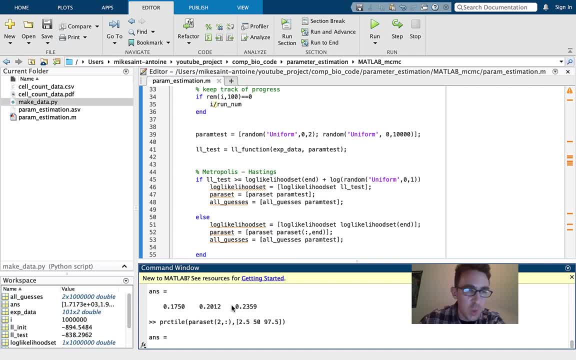 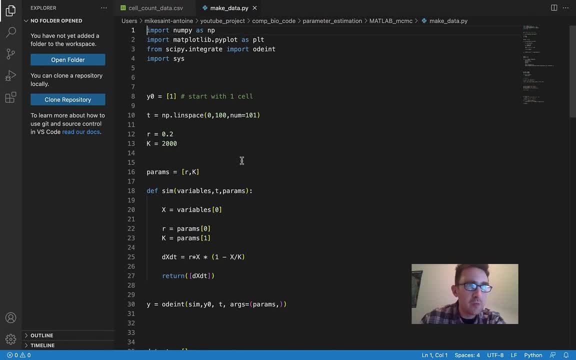 um came pretty close to getting it right. It's not not a hundred percent exact, but uh, you know it came pretty close to getting it right, Um. so yeah w we were able to successfully um recover these parameters that were used to generate this stochastic data.